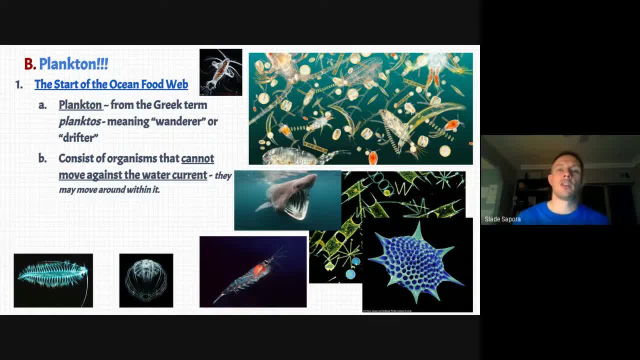 in the current, but they can't just go against it, such as larger things like fishes and whales, et cetera. Plankton is the life of ocean organisms Spend part of their life as plankton, And this is differs from another term that we would then use, called nectin. Nectin would be those larger. 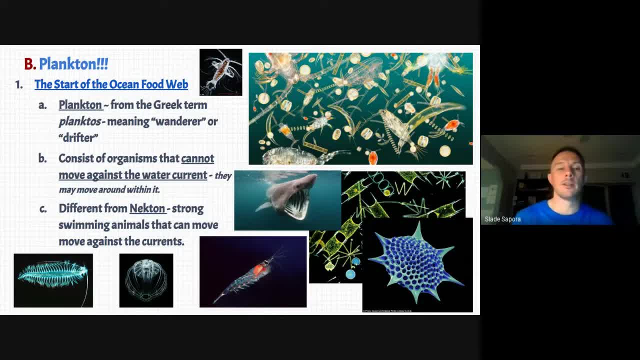 organisms that are stronger, that can actively swim against the current. Okay, So that's definitionally what plankton is And again, generally we're talking about microscopic things that are hard to see with just your eye. Normally we would do a lab where we would look at 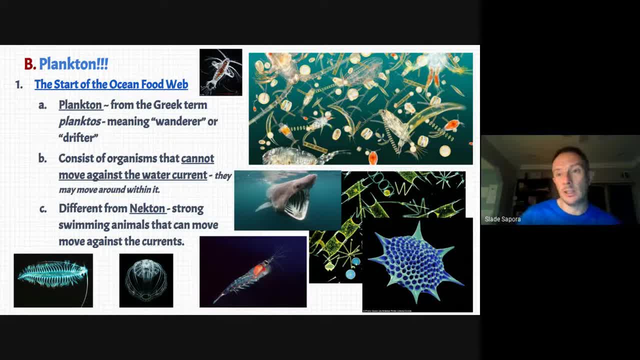 microscopes for a couple of days. Sorry, I'm going to have to leave that one out, But you can see here kind of some of the different things that we'd be looking at if we did look under a microscope, And actually this image right here is a great representation of things that we see commonly. 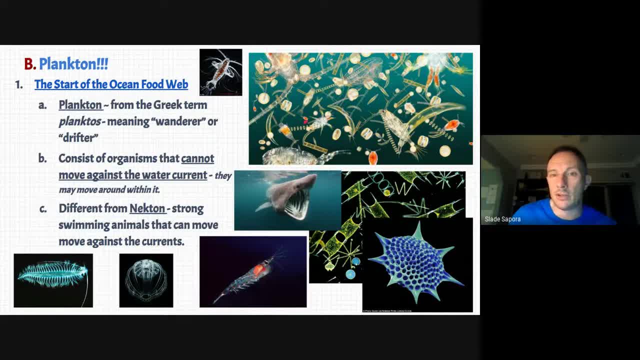 just here in our water, The tinier things that you're seeing here, the little chains of things- these are diatoms and these are photosynthetic forms of algae- almost that we'll be talking about here in a minute. And then the larger ones here with the little antenna: these are copepops. 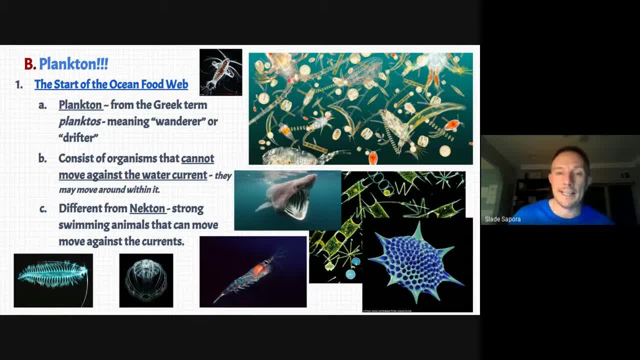 probably the most numerous animal on the planet. And then, of course, you've got things like nectin over here, this giant basking shark, and these things are plankton eaters as well. The largest things in the world are plankton eaters, and including whales, because there's so much plankton. 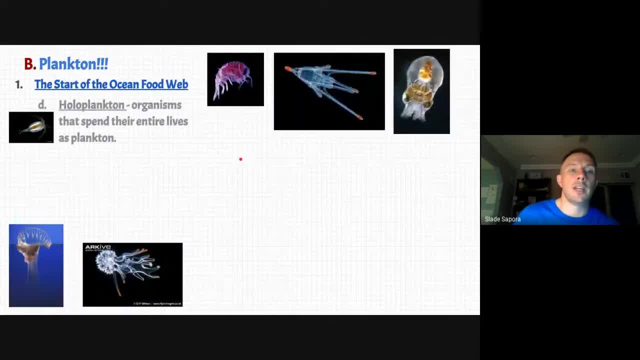 out there, All right, next slide. So again, it is the start of the ocean food wave. Okay, great. So two different types of plankton that we can classify plankton into- I guess would be the way to look at it- Holoplankton. 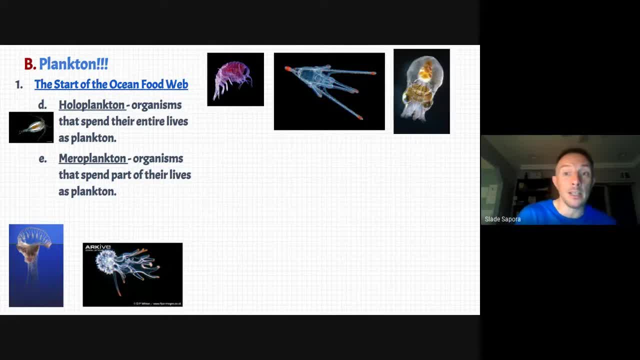 they're organisms that spend their whole entire life as plankton. So every stage of their life cycle they're plankton. And things you could think about there- holoplankton, jellyfish On the big scale- they're plankton their whole life. Copepods, some of these little shrimp and 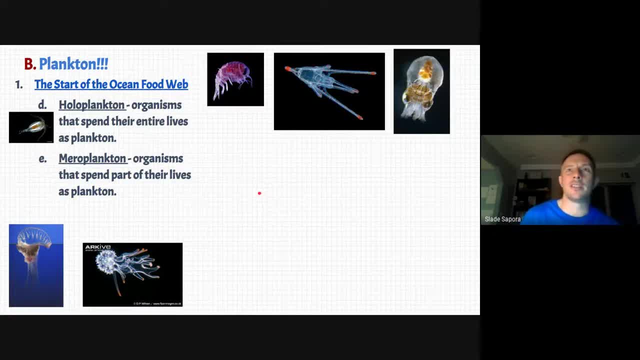 krill, of course. photosynthetic algaes and things like that, like diatoms that are single-celled, are plankton their whole life. Meroplankton are organisms that just spend part of their life as plankton. So holoplankton are organisms that just spend part of their life as plankton. So 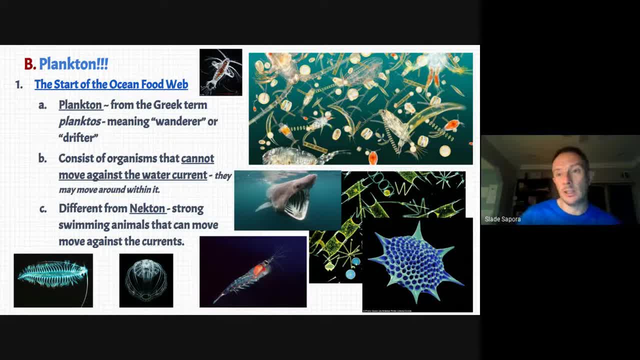 microscopes for a couple of days. Sorry, I'm going to have to leave that one out, But you can see here kind of some of the different things that we'd be looking at if we did look under a microscope, And actually this image right here is a great representation of things that we see commonly. 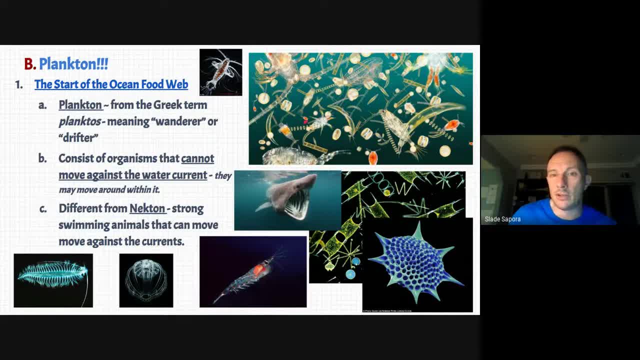 just here in our water, The tinier things that you're seeing here, the little chains of things- these are diatoms and these are photosynthetic forms of algae- almost that we'll be talking about here in a minute. And then the larger ones here with the little antenna: these are copepops. 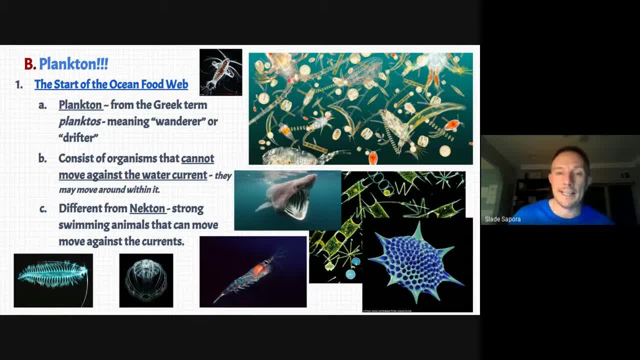 probably the most numerous animal on the planet. And then, of course, you've got things like nectin over here, this giant basking shark, and these things are plankton eaters as well. The largest things in the world are plankton eaters, and including whales, because there's so much plankton. 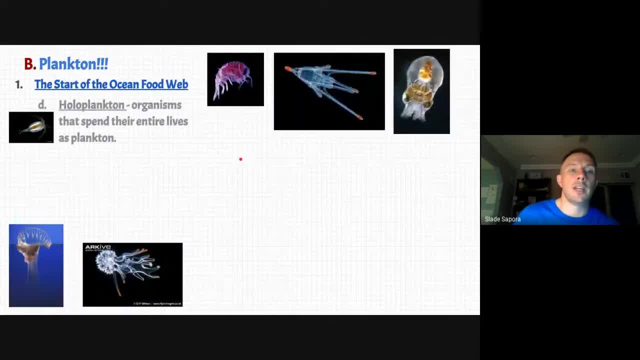 out there, All right, next slide. So again, it is the start of the ocean food wave. Okay, great. So two different types of plankton that we can classify plankton into- I guess would be the way to look at it- Holoplankton. 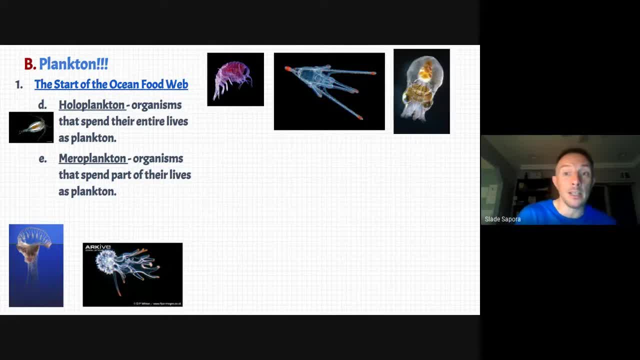 Holoplankton are organisms that spend their whole entire life as plankton, So every stage of their life cycle they're plankton. And things you could think about there- holoplankton, jellyfish On the big scale- they're plankton their whole life. Copepods- some of these little shrimp and 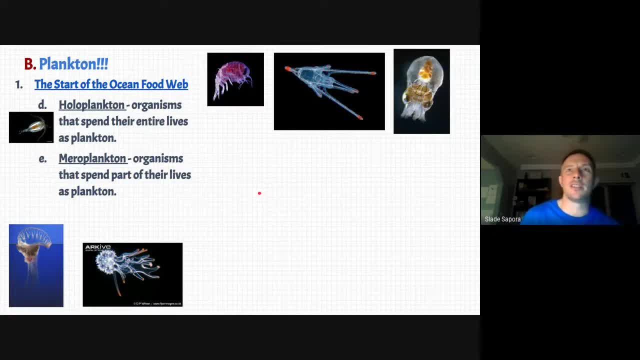 krill, of course. photosynthetic algaes and things like that, like diatoms that are single-celled, are plankton their whole life. Meroplankton are organisms that just spend part of their life as plankton. So holoplankton are organisms that just spend part of their life as plankton. So 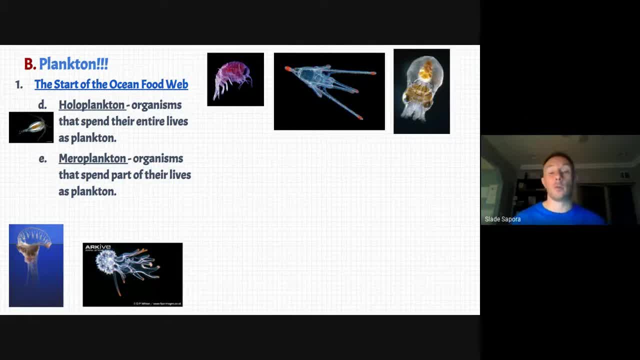 usually it's like a larval stage and there's a whole ton of organisms that do this in the ocean. In fact, most things that we think about or that we see kind of attached to rocks have a life cycle where they're free-floating as plankton when they're younger- Mussels, clams, sea anemones. 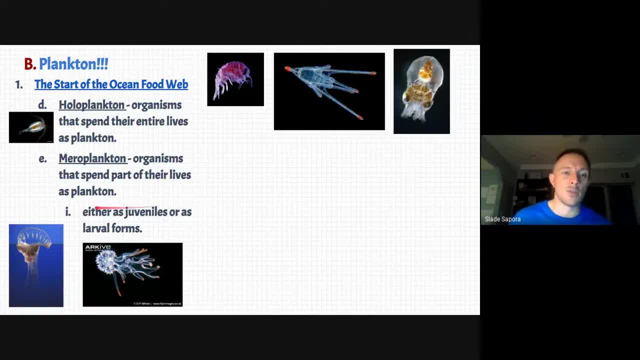 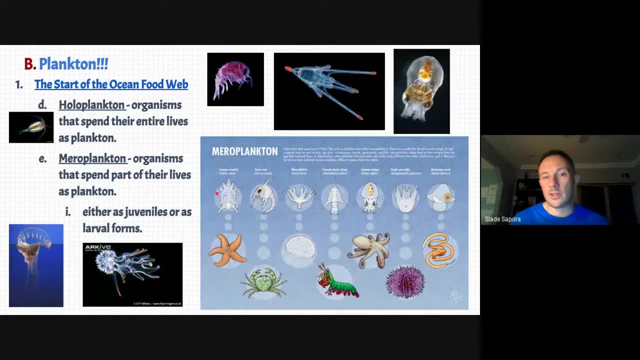 starfish, sea stars, all these other things have planktonic stages when they're young, juvenile larval forms, And for meroplankton here they're a kind of a cool little chart that I found that shows some of the different stages. 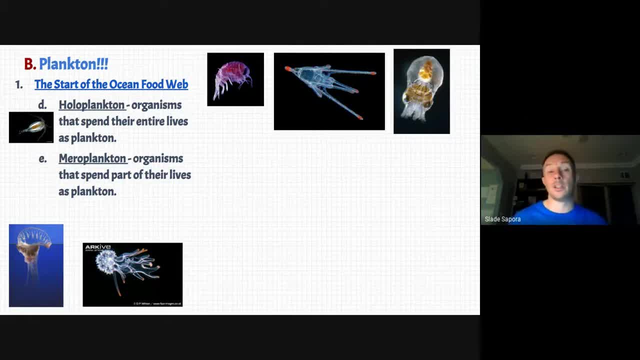 usually it's like a larval stage and there's a whole ton of organisms that do this in the ocean. In fact, most things that we think about or that we see kind of attached to rocks have a life cycle where they're free-floating as plankton, when they're younger, Mussels, clams. 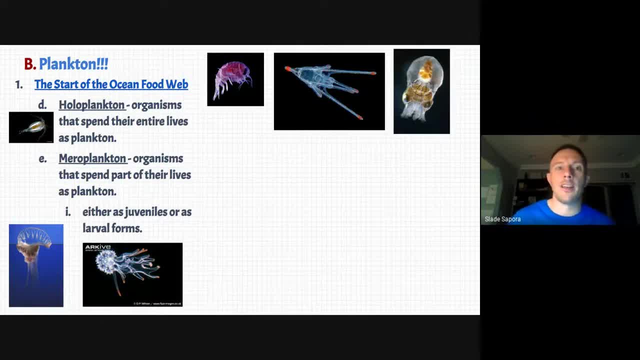 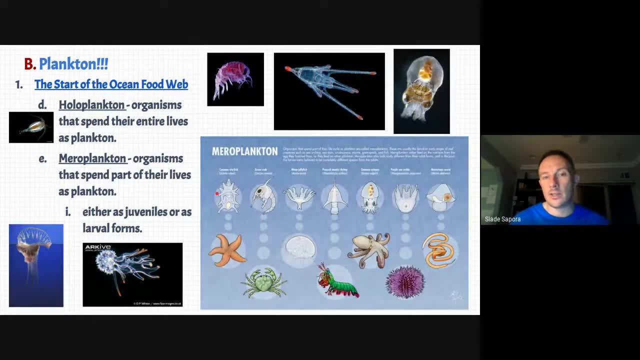 sea anemones, starfish sea stars, all these other things have planktonic stages when they're young, juvenile larval forms, And for meroplankton here there's kind of a cool little chart that I found that shows some of the different stages. 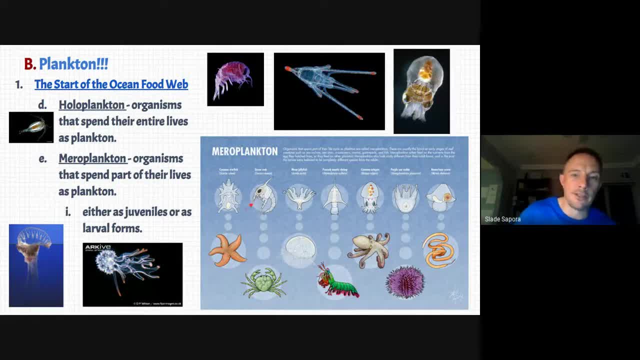 Interestingly enough, I just noticed there's a flaw in here. Anyway, I'll bring that up in a second. see if you could figure out what it is. The common starfish. here we go, big old starfish you can find in a tide pool. This is what it looks like as a planktonic stage Crab have a plankton. 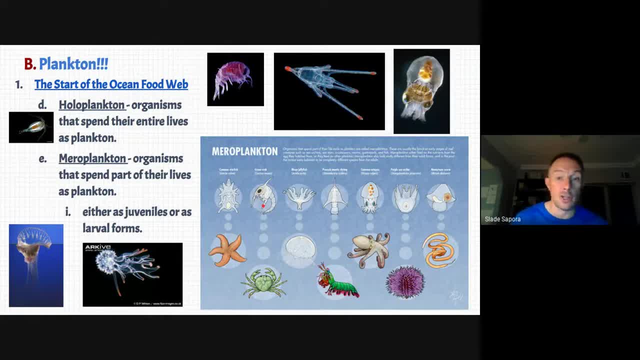 stage as well, when they're larval juveniles. So they float around in the ocean and then they eventually more can grow into larger species. So that's kind of a cool little chart that I found. And then we got the mantis shrimp here. Octopus have a planktonic stage as well. They're really 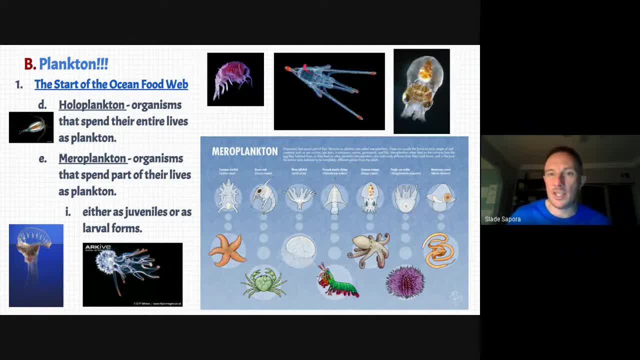 cute looking. We've seen those in our class- Sea urchins. this is a sea urchin right up here, right? Yeah, exactly, They have a plankton stage And then worms and other things like that. So most 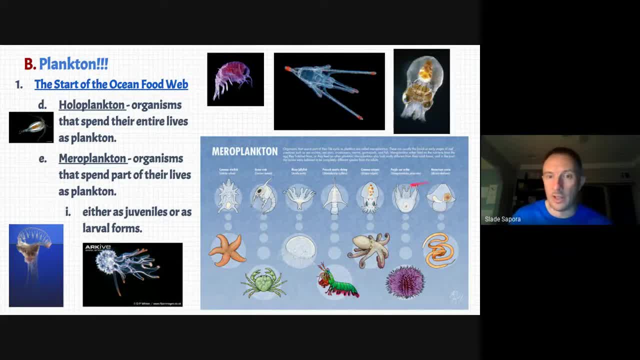 of your invertebrates. things without backbones have a planktonic stage. The one thing that I would say that is not meroplankton here would be the moon jelly. I think this is wrong. Yes, it has a planktonic stage. It's different, But it's a planktonic stage. It's a planktonic stage. 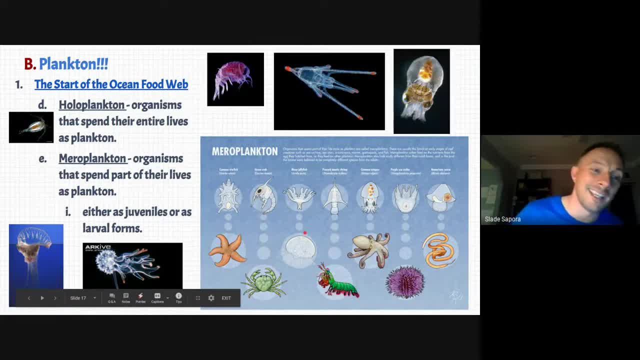 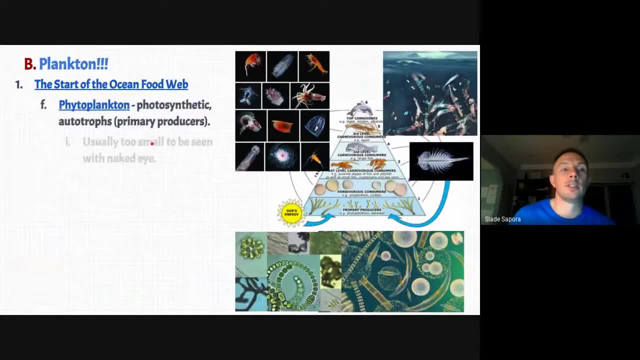 It's different from the adult, but both are actually still plankton. Anyway, that's me being picky, Okay. So at the very base of the ocean food web, at the base of any food web, are your primary producers, right? Your things that do some sort of synthesis of non-organic material into 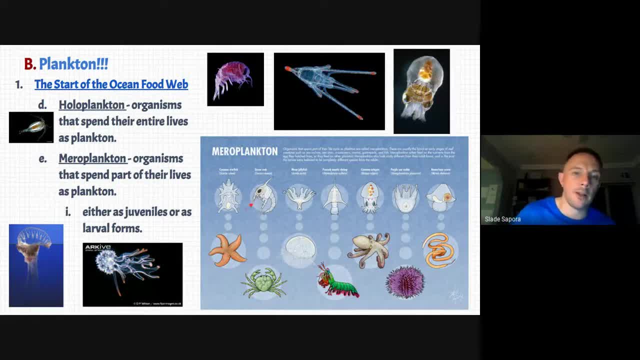 Interestingly enough, I just noticed there's a flaw in here. Anyway, I'll bring that up in a second. see if you could figure out what it is. The common starfish. here we go, big old starfish you can find in a tide pool. This is what it looks like as a planktonic stage Crab have a plankton. 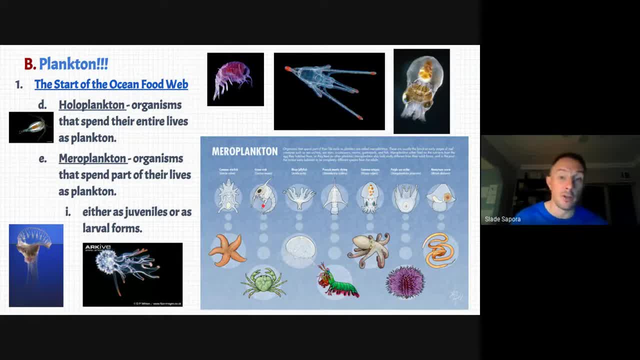 stage as well, when they're larval juveniles. so they float around in the ocean and then they eventually morph and grow into larger forms. So they're a kind of a cool little chart that I found out. And then we got the mantis shrimp here. Octopus have a planktonic stage as well. They're. 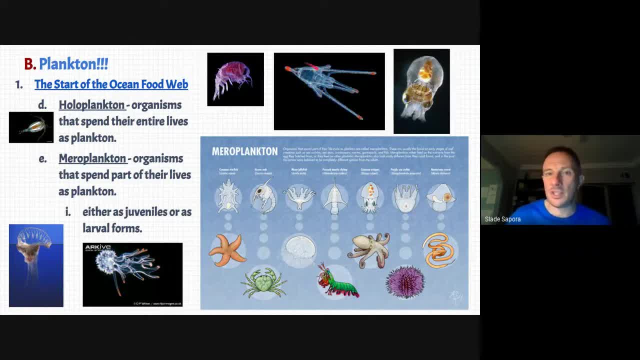 really cute looking. We've seen those in our class: Sea urchins. this is a sea urchin right up here, right? Huh, Yeah, exactly, They have a plankton stage And then worms and other things like that. So most of your invertebrates- things without backbones, have a planktonic stage. 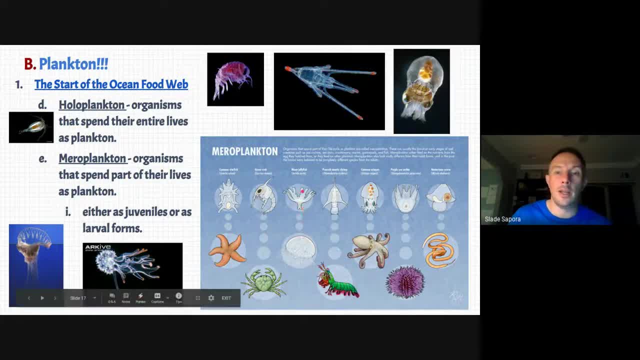 The one thing that I would say that is not meroplankton here would be the moon jelly. I think this is wrong. Yes, it has a planktonic stage. It's different from the adult, but both are actually still plankton. Anyway, that's me being picky. 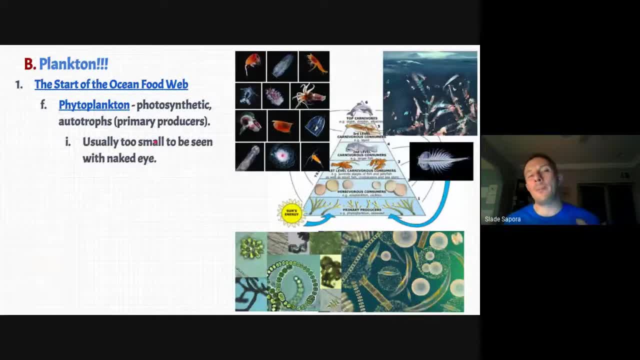 Okay, So at the very base of the ocean food web, at the base of any food web, are your primary producers, right? Your things that do some sort of synthesis of non-organic material into organic material. Generally, we think of this as photosynthesis. 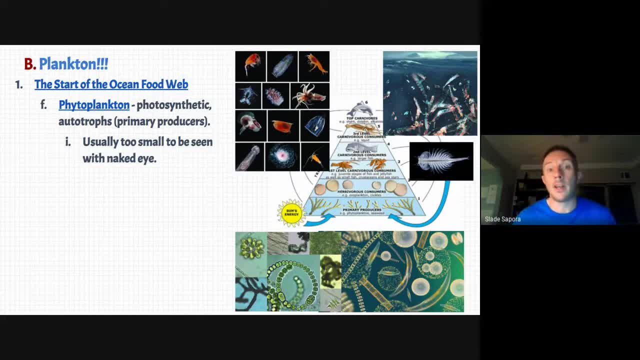 because that's the majority of biological synthesis that goes on Here on planet Earth. there are those weird little chemo-autotrophs we call them, and they do synthesis down at the bottom of the ocean, but they're using chemicals from. 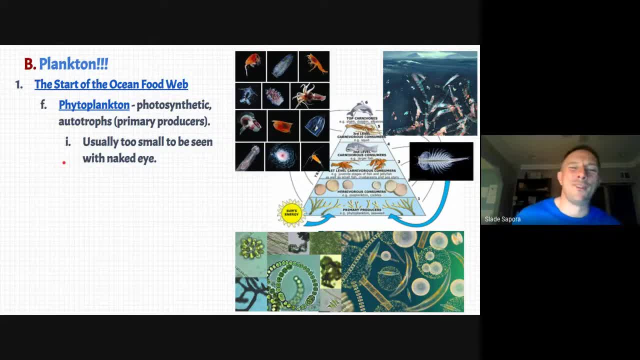 hydrothermal heads. Anyway, we're talking about phytoplankton here, and these are photosynthetic small autotrophs, primary producers, and they sit at the bottom of the ocean food web. They are the base of the ocean food web. They are the forest, the grass, the savanna of the sea, so to speak. 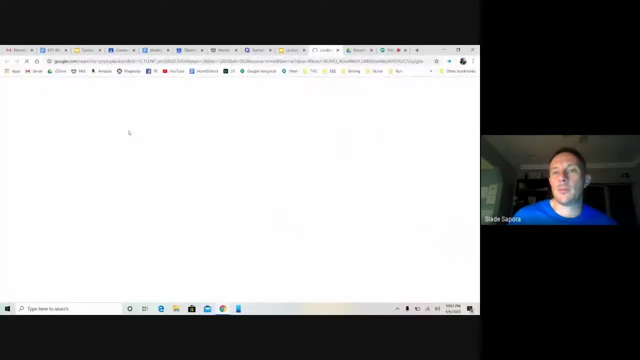 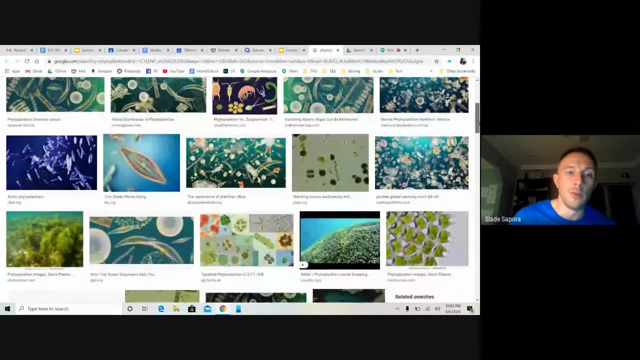 And I have a link here, so I'm curious to see where this will take us. Oh, here's just some different images, All the different images of phytoplankton. They're really really cool and beautiful looking. Many of them have these really elaborate cell walls that they make. 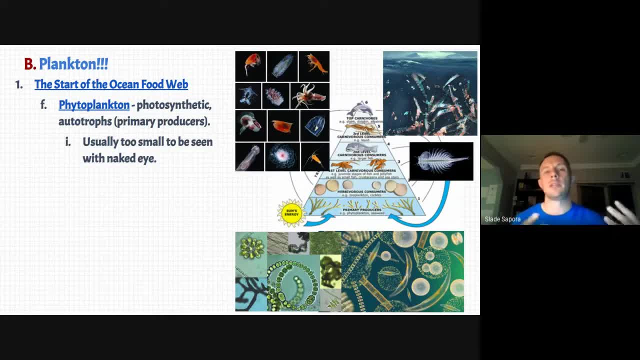 organic material. Generally we think of this as photosynthesis, because that's the majority of biological synthesis That goes on here on planet Earth. There are those weird little chemo-autotrophs we call them, And they do synthesis down at the bottom of the ocean, but they're using chemicals from. 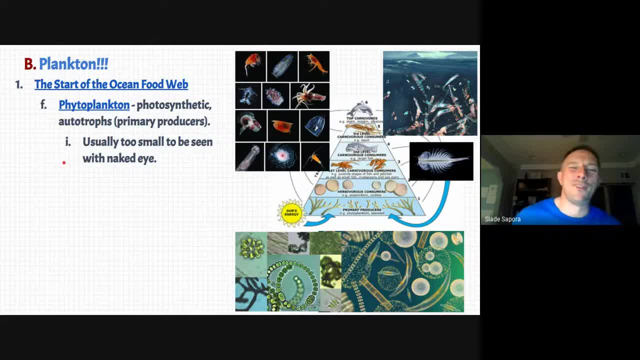 hydrothermal heads. Anyway, we're talking about phytoplankton here, And these are photosynthetic small autotrophs, primary producers, and they sit at the bottom of the ocean food web. They are the base of the ocean food web. They are the forest, the grass, the savanna of the sea. 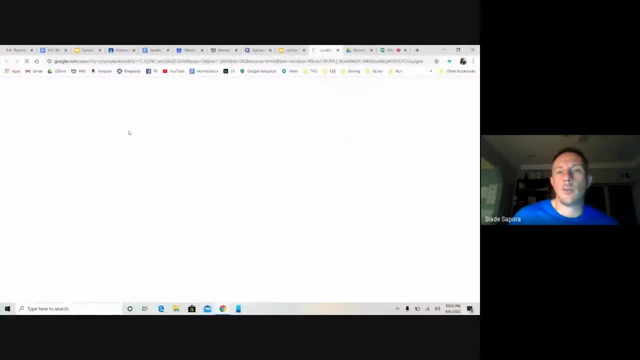 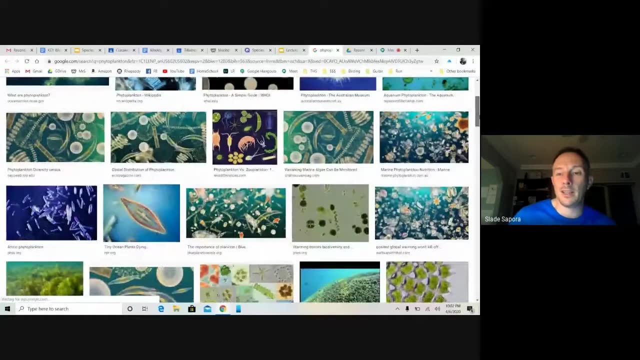 so to speak, And I have a link here. so I'm curious to see where this will take us Probably. Oh, here's just some different images, all the different images of phytoplankton. They're really really cool and beautiful looking. Many of them have these really elaborate cell walls. 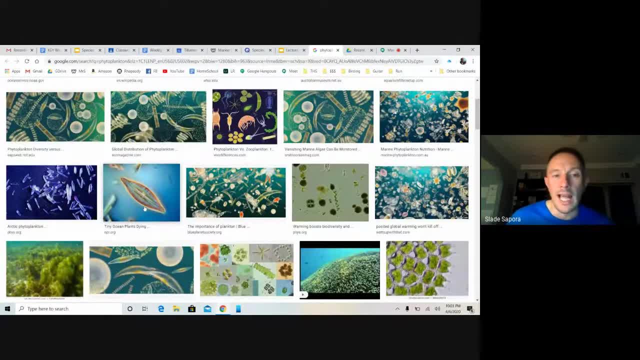 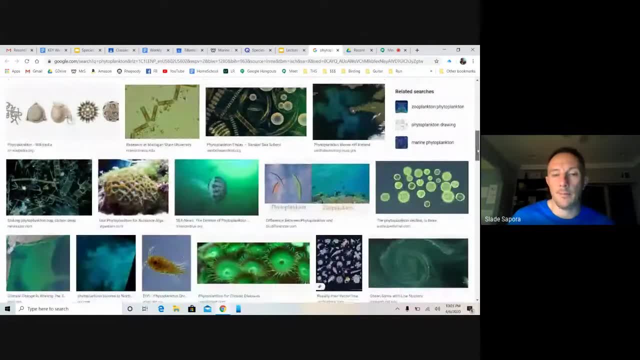 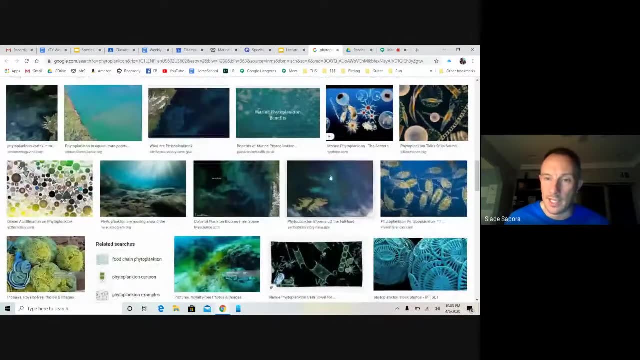 that they make. They're single-celled still, but they have these cell walls made of glass or cellulose, depending on the type of phytoplankton that you're looking at, And microscopically they just They're just cloud up the ocean and you can see big blooms of them from space. You can see that. 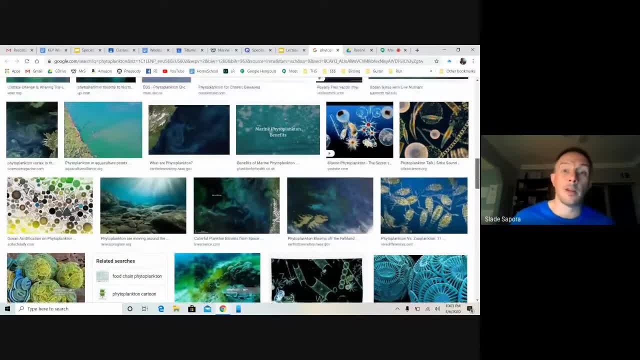 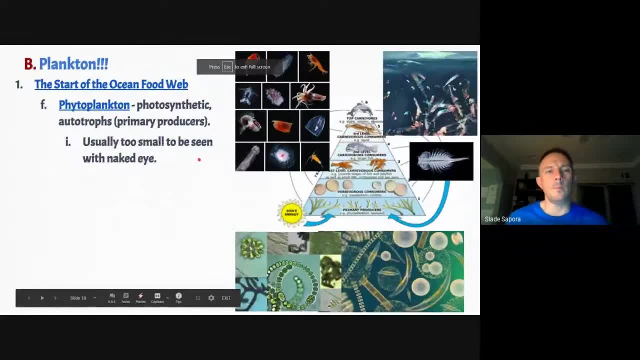 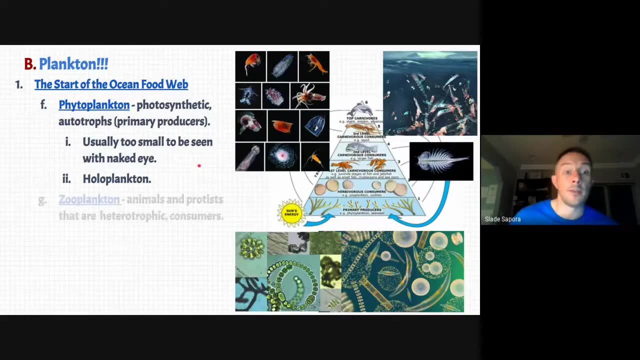 here, And they also make our red tide in the summertime here as well. the dinoflagellates: Get so many of those. Okay, bring this back up. Cool Again, usually too small to be seen with the naked eye. No death, Holoplankton. I mean they spend their whole life as plankton, Okay. 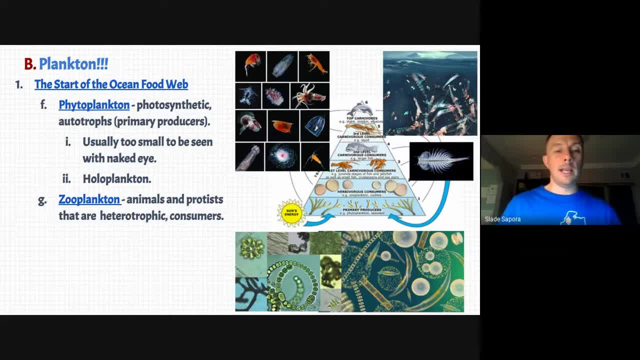 Zooplankton are the other type of plankton that we could be talking about, And they generally consist of animals belonging to the animal kingdom, such as crustaceans, shrimps, jellyfish, things of that nature and all the different larval stages, And then protists. 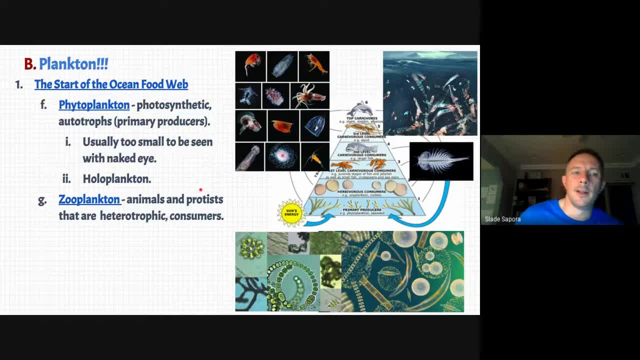 which would be sort of single-celled heterotropes, Consumers, things that do not do photosynthesis but they eat things. There's a whole host of those too: Zooplankton, range in size from microscopic up to jellyfish, which you can see, And 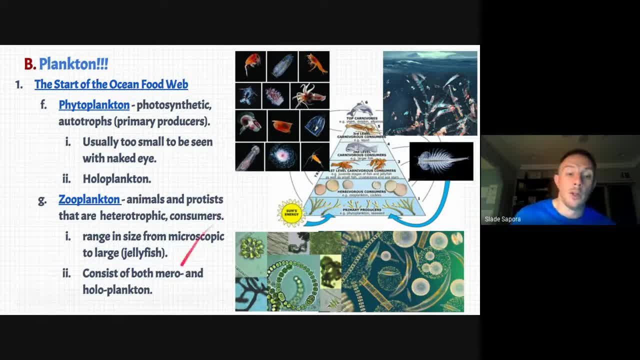 They consist of both marrow and holoplankton. So there are those things that just spend part of their life as zooplankton- the larval stages of sea, anemones, crabs and various other organisms- And then they later go on to become non-plankton, where they settle on the bottom of the ocean. So 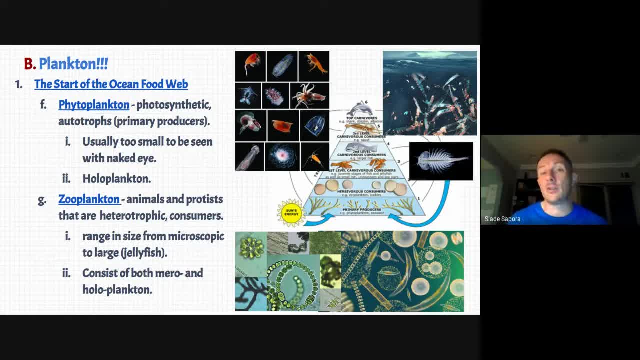 if you're not drifting in the ocean, you're not plankton right, You're attached to the bottom. That's another type of organism we'll talk about later, called benthic. in case you were wondering, Okay, And here's just. 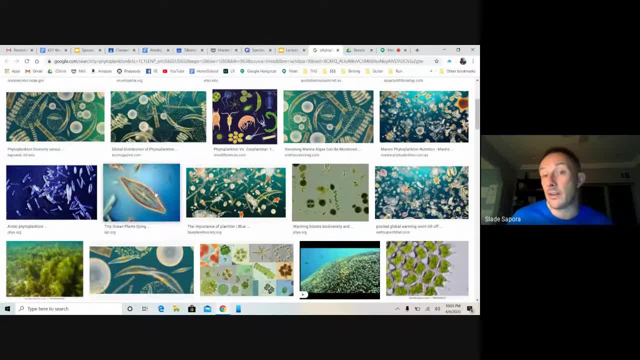 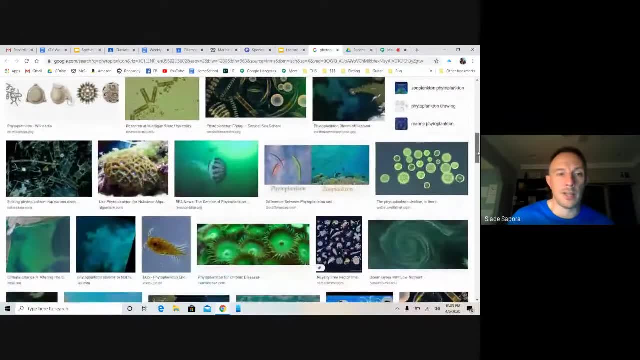 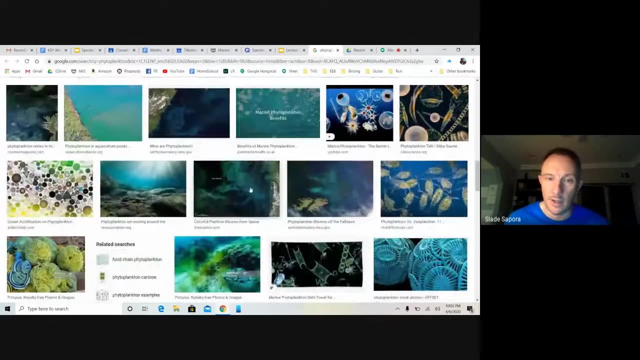 They're single-celled still, but they have these cell walls made of glass or cellulose, depending on the type of phytoplankton that you're looking at, and microscopically they just cloud up And you can see big blooms of them from space. You can see that here And they also make our red tide. 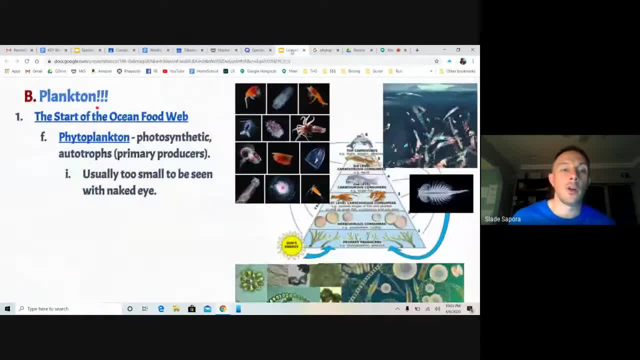 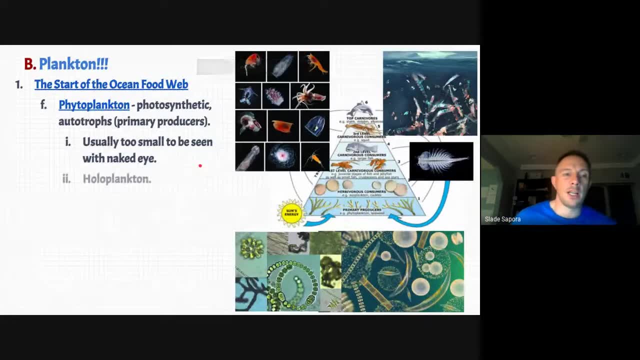 in the summertime here as well. the dinoflagellates: You get so many of those. Bring this back up. Cool Again, usually too small to be seen with the naked eye. No death, Holoplankton. I mean, they spend their whole life as plankton. 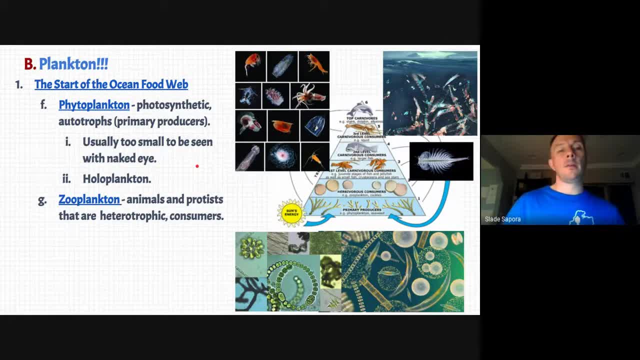 Okay, Zooplankton are the other type of plankton that we could be talking about, and they generally consist of animals belonging to the animal kingdom, such as crustaceans, shrimps, jellyfish, things of that nature and all the other larval stages, And then protists. 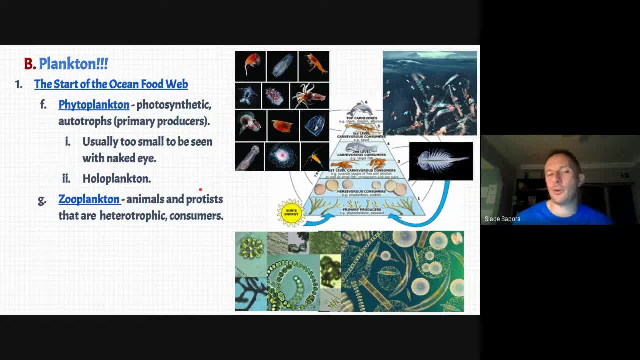 which would be sort of single-celled heterotropes, Consumers, things that do not do photosynthesis but they eat things. There's a whole host of those too: Zooplankton range in size from microscopic up to jellyfish, which you can see. 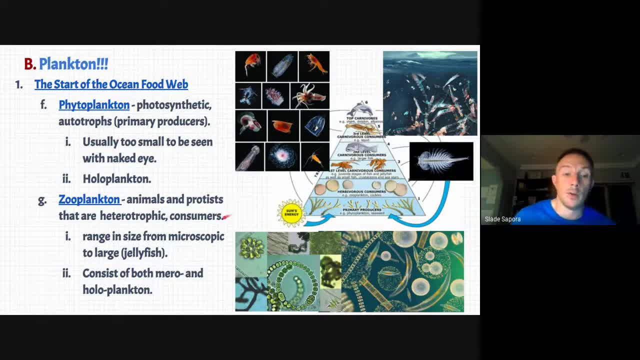 And they consist of Both marrow and holoplankton. So there are those things that just spend part of their life as zooplankton- the larval stages of sea, anemones and crabs and various other organisms- And then they later go on to become non-plankton, where they settle on the bottom of the ocean. 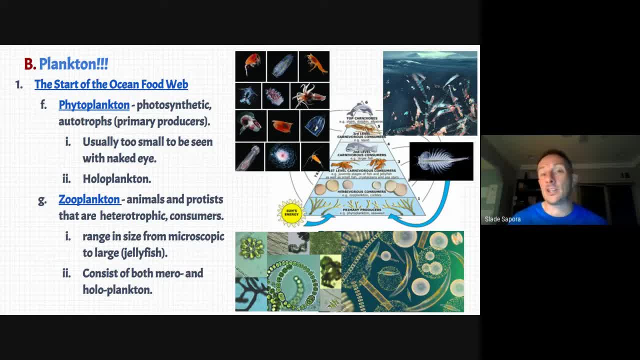 So if you're not drifting in the ocean, you're not plankton right, You're attached to the bottom. That's another type of organism we'll talk about later, called benthic, in case you were wondering. Okay, And here's just a. 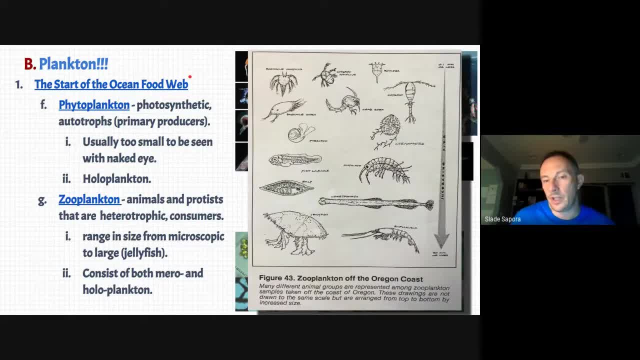 little image showing some of the zooplankton that we have off of the Oregon coast. here Some pretty cool drawings Again: fish, larvae, Barnacles spend part of their life as plankton before they anchor onto rocks. Copepods spend their hololife as plankton before their holoplankton. 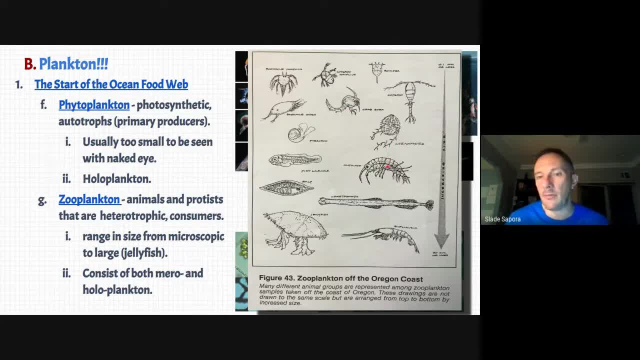 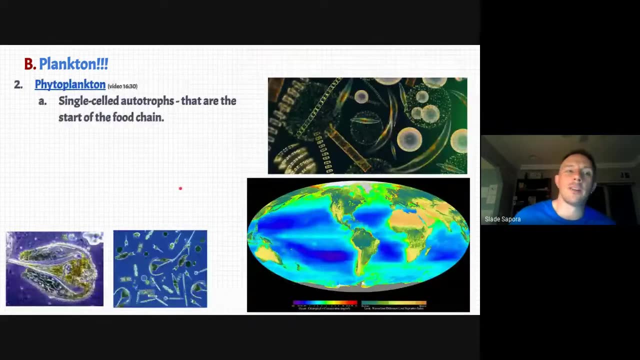 Here's another copepod. there There's crab larvae, And amphipods are similar to shrimp. They're actually roly polies. A lot of types of amphipods on land are another one sort of similar to shrimp as well. Okay, Moving along, Let's talk about phytoplankton. 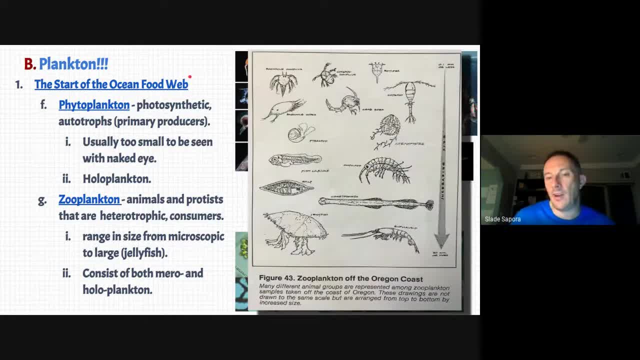 Just an image showing some of the zooplankton that we have off of the Oregon coast. here Some pretty cool drawings Again: fish larva Barnacles spend part of their life as plankton before they anchor onto rocks. Copepods spend their hololife as plankton before they're. 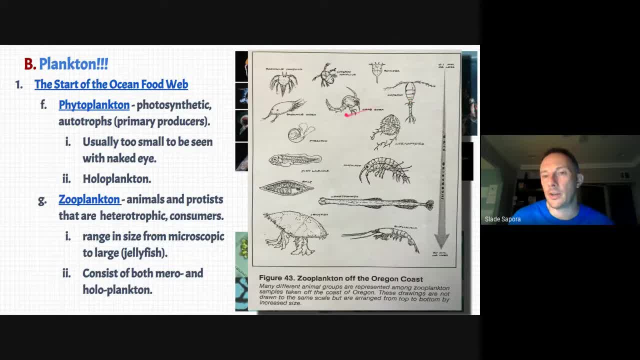 holoplankton. Here's another copepod there. Here's a crab larva And amphipods are similar to shrimp. They're actually roly-polies are a type of amphipod on land. Euphazids are another one sort of similar to shrimp as well. 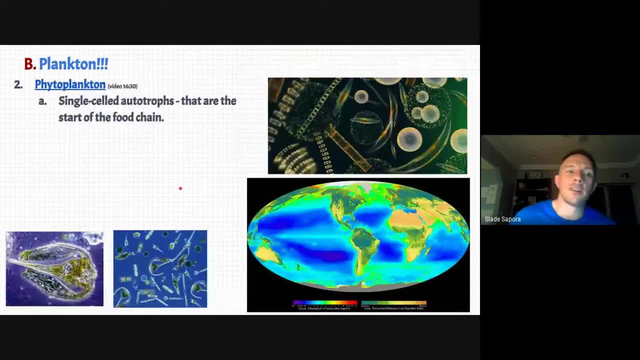 Okay, Moving along, Let's talk about phytoplankton. There's a hyperlink here to a video I have and you can check that out. Looks like there's a section on phytoplankton that starts at minute 16, second 30 there, So you can advance to that. I believe this is the Planet Ocean video. 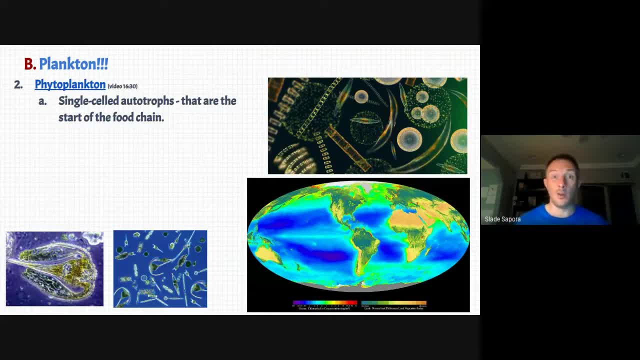 It's a really cool documentary. You should watch the whole thing. right, You're stuck at home might as well. Okay, Phytoplankton are. They are generally single-celled autotrophs, meaning that they do make their own food. 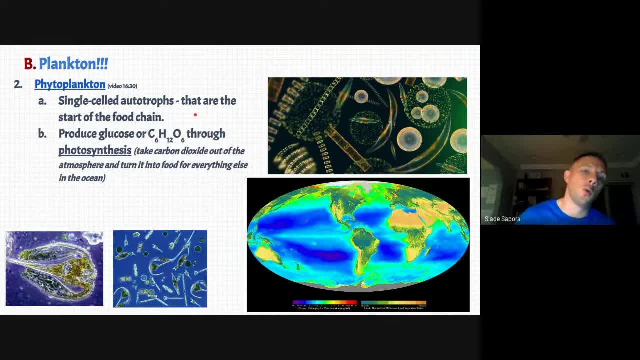 And they are the start again, of every ocean food chain. It's more important than just saying they're the start of the ocean food chain. Really think of them as being those primary producers that make glucose, that make sugar, that take the inorganic. 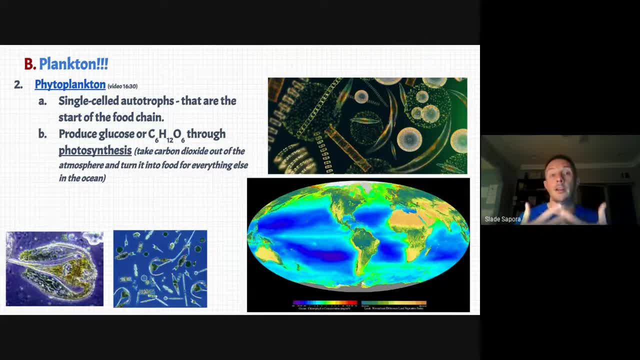 carbon dioxide and water and turn it into the organic C6H12O6.. Know your Cho What's up? Cho Oh Cho. Okay, And they do this through photosynthesis. Boom. And as a byproduct to making all of this sugar and food for themselves, they give off a lot of oxygen. 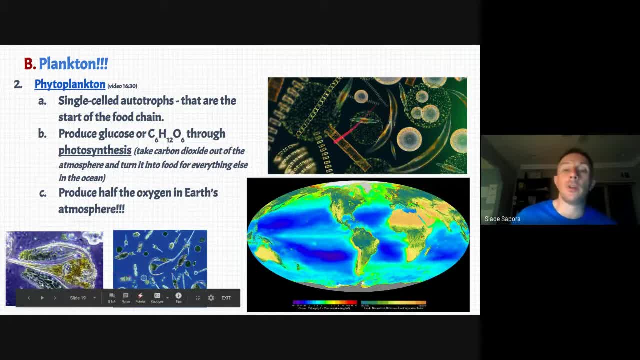 About half the earth's oxygen is given off and exhaled by these organisms as they're making sugar. This little map down here. Do I have it blown up in the next slide? Let me see Woohoo, why here? Okay, Why to get down there? Why do we see the map for all the way to the Phytoplankton? 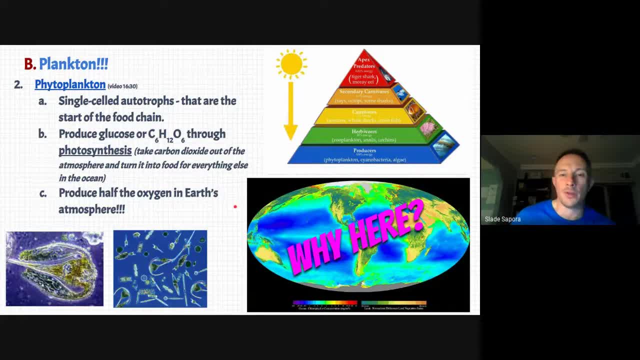 Okay, Why be so good at Gmail? Okay, I don't know. Yeah, Every first week on me, first and every second, I'm thinking about Google on my desk, while I'm never lightweight. see them in the places that we see them. Why do we see these primary producers? And I'm going to 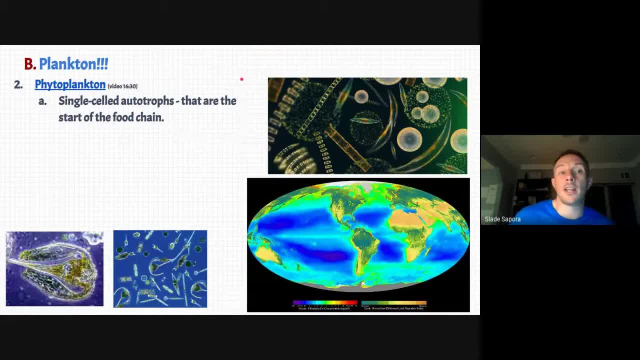 There's a hyperlink here to a video I have And you can check that out. Looks like there's a section on phytoplankton that starts at minute 16, second 30 there, So you can advance to that. I believe this is the planet ocean video. It's a really cool documentary. You should watch the. 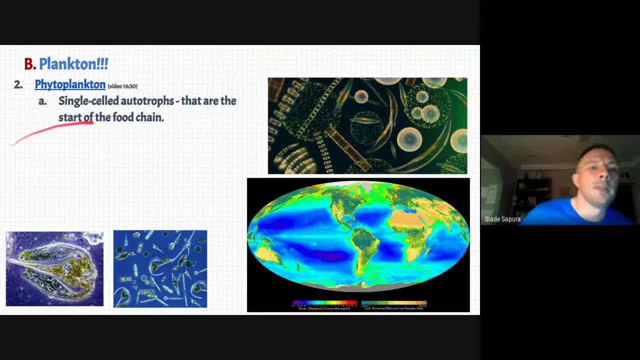 whole thing right. You're stuck at home, Might as well. Okay. Phytoplankton are generally single cell autotrophs, meaning that they do make their own food And they are the start again of every ocean food chain. It's more important than just saying they're the start of the ocean food chain. 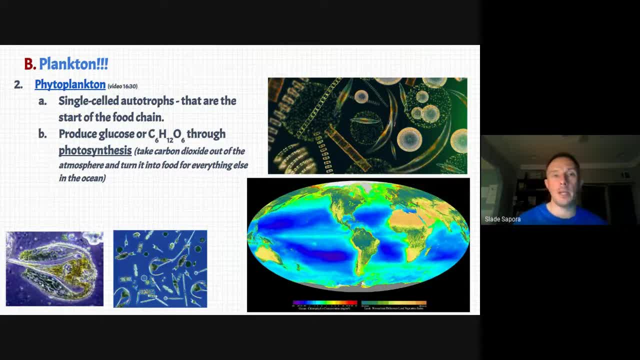 Really think of them as being those primary producers that make glucose, that make sugar, that take the inorganic carbon dioxide and water and turn it into the organic C6H12O6.. Know your Cho What's up Cho Oh, Cho Okay. 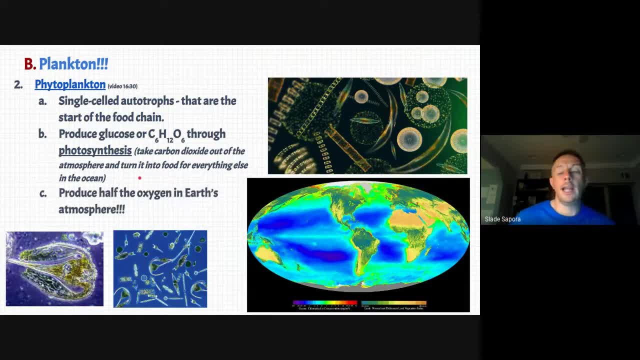 And they do this all the time. this through photosynthesis Boom. And as a byproduct to making all of this sugar right and food for themselves, they give off a lot of oxygen. About half the earth's oxygen is given off and exhaled by these organisms as they're making sugar. This little map down here, do I? 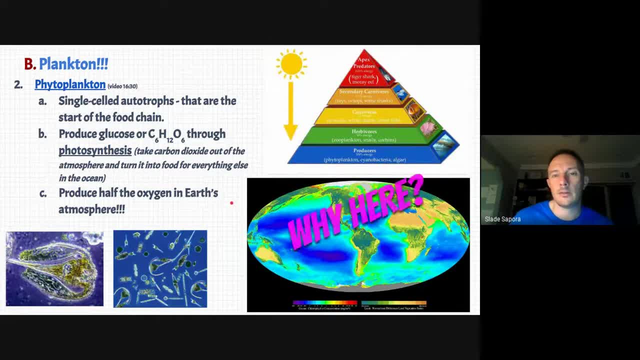 have it blown up on the next slide. Let me see Why here. Okay, Why do we see them in the places that we see them? Why do we see these primary producers- And I'm going to have to back that up then, Hang on just a second- Why do we see them in the zones that we see them? If you're looking, 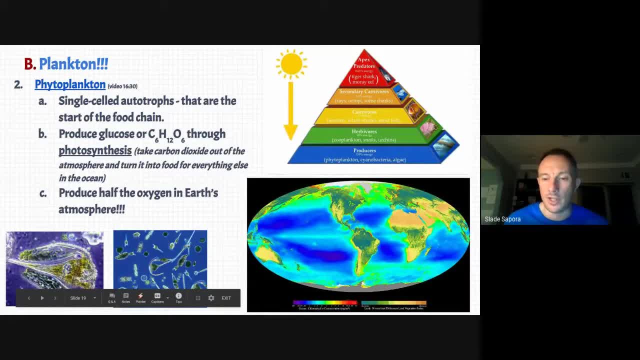 at this map down here, the highest concentrations of photosynthetic organisms are in red, The lowest concentrations are in purple. So what's weird is that the middle sections of the ocean right both in the North Pacific and the South Pacific, these sort of areas that correspond to 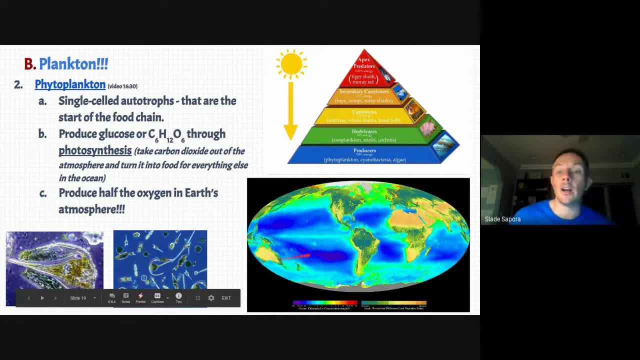 high concentrations of photosynthetic organisms are in red. So what's weird is that the middle sections of the ocean are red. So what's weird is that the middle sections of the ocean are in purple. So this is the tropic of cancer, This is the tropic of Capricorn, our dead zones in the ocean, And 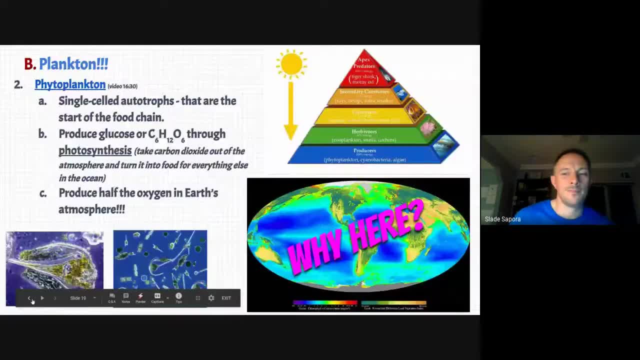 have to back that up. then Hang on just a second. Why do we see them in the zones that we see them? If you're looking at this map down here, the highest concentrations of photosynthetic organisms are in red, The lowest concentrations are in purple. So what's weird is that the middle. 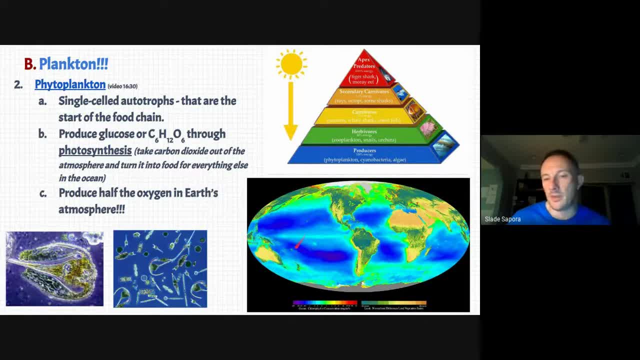 sections of the ocean right, both in the North Pacific and the South Pacific. these sort of areas that correspond to high pressure dry air- this is the Tropic of Cancer, this is the Tropic of Capricorn- are dead zones in the ocean. And they're kind of dead zones in the ocean because 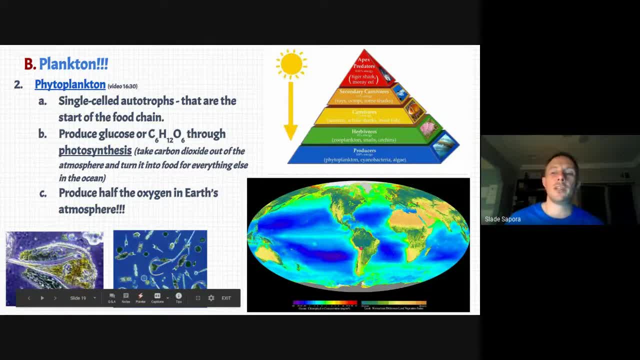 there's really no wind there, And so there's nothing to carry nutrients from land out into the ocean. There's no currents ripping through here. Now there's a huge current that rips along the equator, right in here, And this is what gives us our trade winds, or our easterly winds as well. 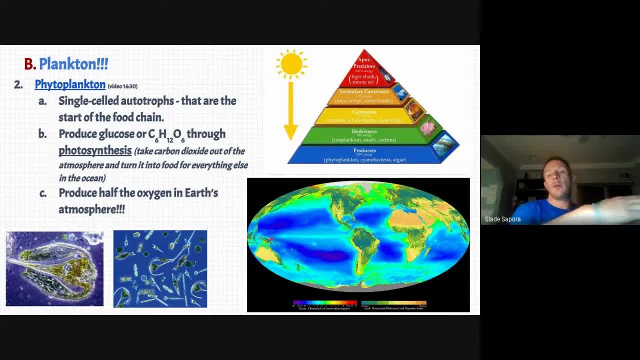 And there's a constant gesture of air just kind of flowing down along the equator And it pushes nutrients from the land, from the Congo, in here and then of course from Ecuador basically in here out across the ocean, And that supplies this plankton with nutrients, fine little minerals. 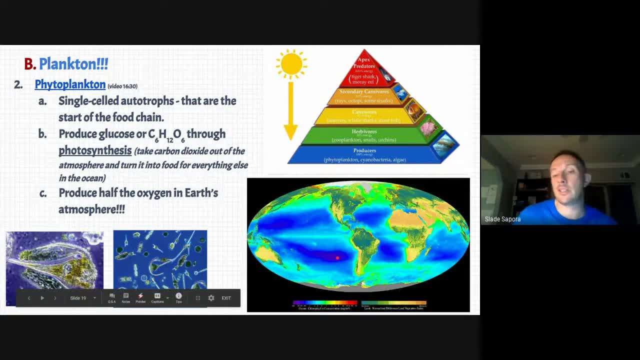 and things like that, from soil Out here there are no nutrients because there's no wind and the ocean is 12,000 feet deep, And so there's this disconnect between the light and the actual nutrients below, So there's not much mixing. 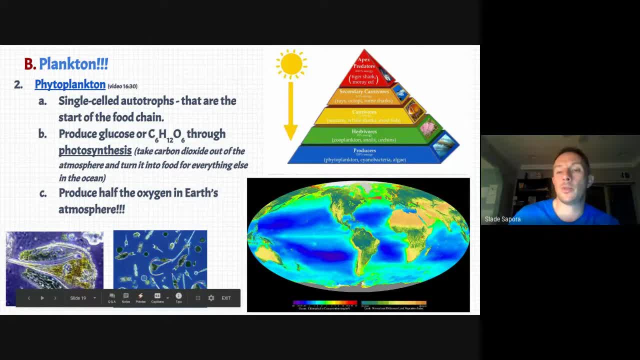 In these areas. the Southern Ocean and, of course, up north and North Pacific, Atlantic and the Arctic are the most productive oceans in the world, And that is seasonal, of course, But in the summertime they get 24 hours of light, A lot of wind, mixing the water with nutrients And 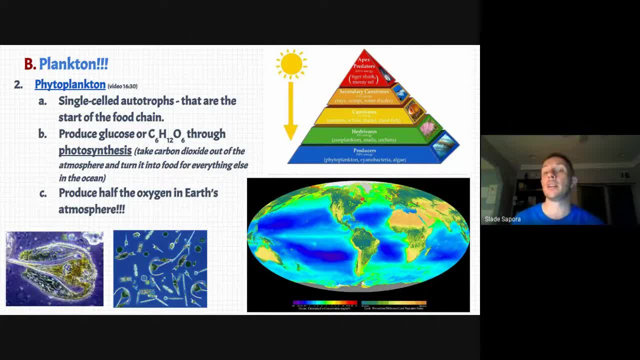 especially in the north, it's very shallow because of the proximity to land, So there's this constant nutrient mixing 24 hours of light. Cold water actually holds more oxygen and it's much more productive in these oceans And it's why whales, birds and so many other things are so. 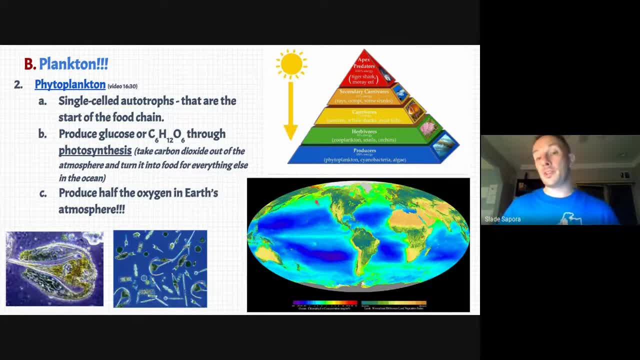 important, And that's why these things migrate to these regions. That's why salmon leave our rivers and head up to Alaska to grow big, Because there's just so much food that gets produced up there seasonally that then other organisms take advantage of that. 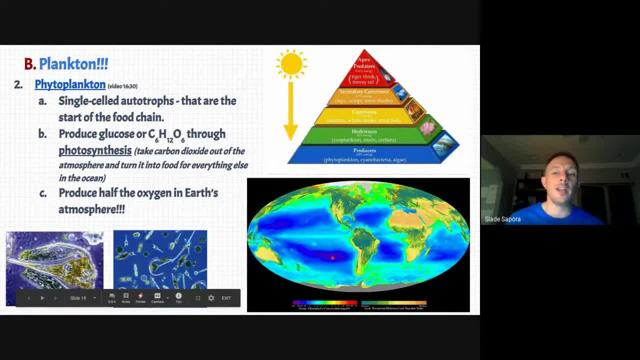 they're kind of dead zones in the ocean, because there's really no wind there And so there's nothing to carry nutrients from land out into the ocean. There's no currents ripping through here. Now there's a huge current that rips along the equator, right in here, And this is what gives us. 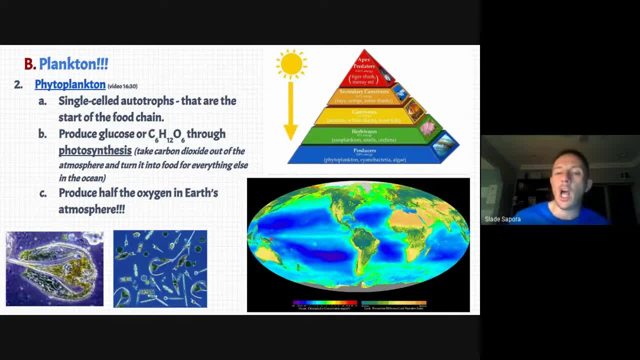 our trade winds or our easterly winds as well, And there's a constant gesture of air just kind along the equator and it pushes nutrients from the land, from the congo in here and then of course from ecuador basically in here out across the ocean, and that supplies this plankton with 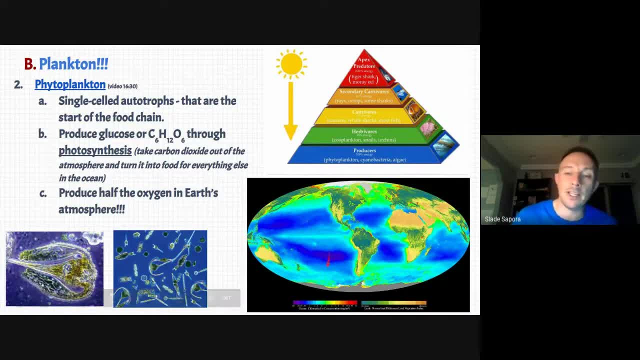 nutrients- fine little minerals and things like that- from soil. out. here there are no nutrients because there's no wind and the ocean is 12 000 feet deep, and so there's this disconnect between the light and the actual nutrients below. so there's not much mixing in these areas. the southern 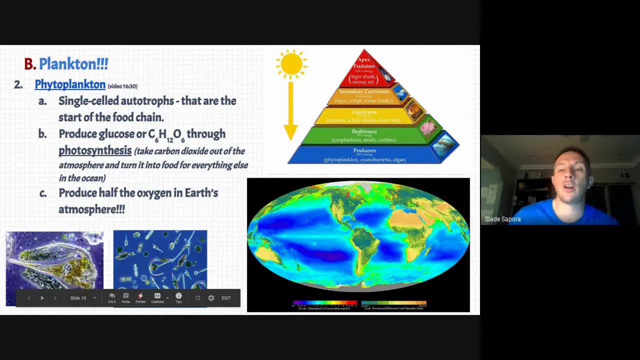 ocean and of course up north and north pacific, atlantic and the arctic are the most productive oceans in the world and that is seasonal, of course, but in the summertime they get 24 hours of light, a lot of wind mixing the water with nutrients and especially in the north it's very shallow because 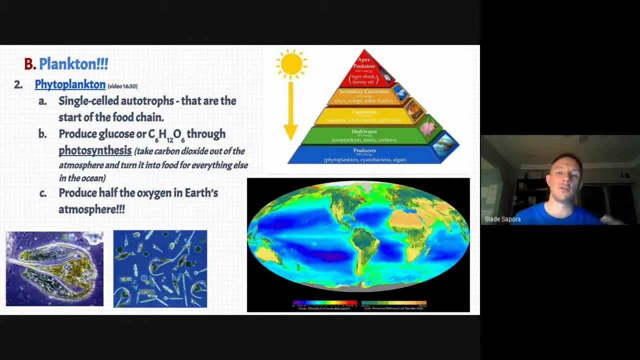 of the proximity to land. so there's this constant nutrient mixing 24 hours of light. cold water actually holds more oxygen and it's much more productive um in these oceans, and it's why whales, birds and so many other things migrate um to the ocean. so that's why they're so important. 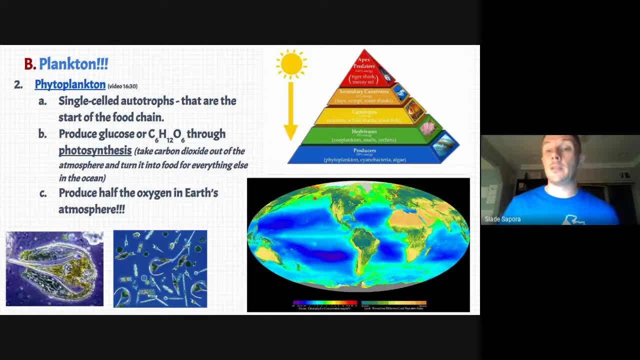 in these regions. that's why salmon leave our rivers and head up to alaska to grow big, because there's just so much food that gets produced up there seasonally that, um then other organisms take advantage of that: cool beans. so while i hear, i think i just answered that. okay, next up. 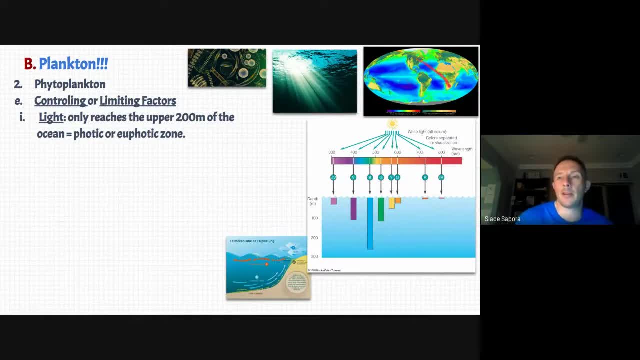 so what is it that controls why we see phytoplankton where we do? again back to this map here showing the why here. why do we see them in the north and in the south, along the equator and then really abundantly along coastlines all around the planet? um, one of the reasons that we see 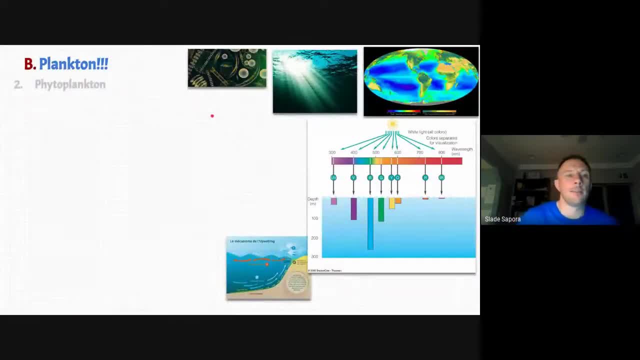 Cool beans. So, while I'm here, I think I just answered that. Okay, next up. So what is it that controls why we see phytoplankton where we do This map here showing the why here? Why do we see them in the north and in the south along the? 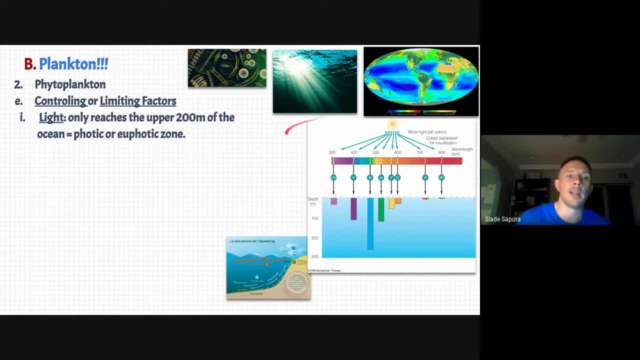 equator and then really abundantly along coastlines all around the planet. One of the reasons that we see plankton where we do is light right. So if you're doing photosynthesis, you need the photo part to do the synthesis. Okay, so light only reaches the upper 200 meters of the ocean in the 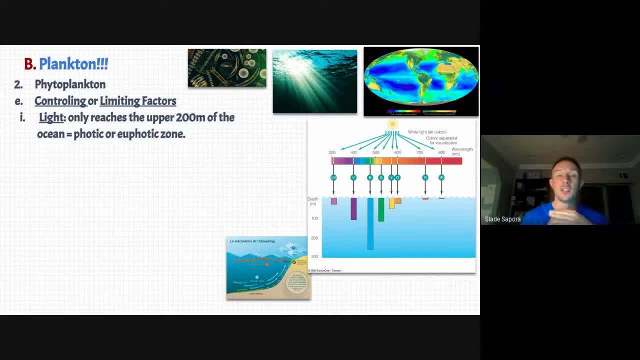 photic zone. Below that 200 meter depth it's 99% of the ocean. So if you're doing photosynthesis, all light is gone- It's what we call the aphotic zone, And so light doesn't penetrate. And this 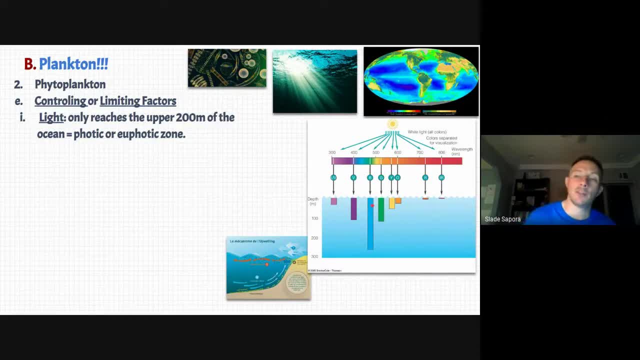 graphic here kind of shows what types of light and penetrate into what depth. right, A red light is penetrates the shallowest- only about 10 meters, 30 feet and it's gone. But your blue light tends to penetrate the deepest And that's why we see the ocean is blue. coincidentally, 90% of all marine. 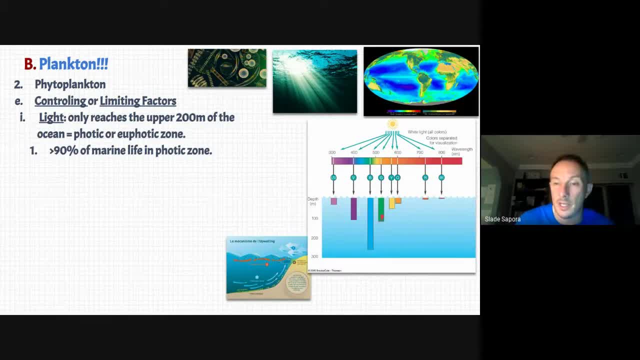 life is in this upper 200 meters. Then this up in here is the photic zone. This is where photosynthesis is happening. So if you're doing photosynthesis, you need to do photosynthesis. So if you're doing photosynthesis below this, no photosynthesis, so not much life at all. And the second thing that 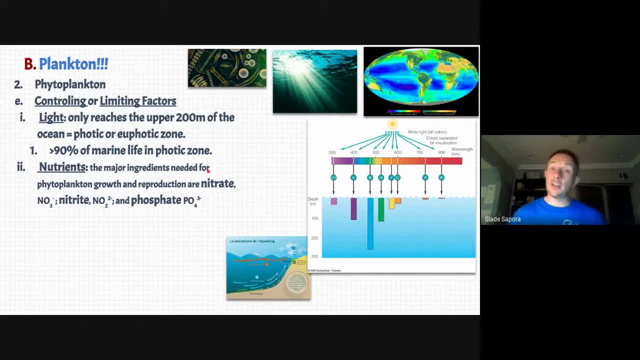 controls or limits where phytoplankton can occur or does occur in abundance is nutrients right? So you've got light penetrating the surface of the ocean in the upper area, But then those nutrients right, The major ingredients that these things need to produce their cells and produce. 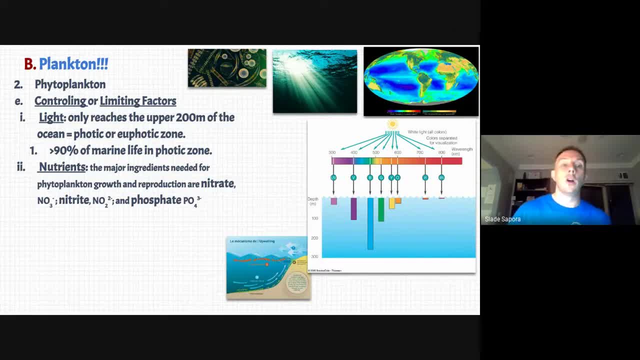 their bodies and make more DNA and blah, blah, blah are nitrates, right nitrogen-containing molecules, and then phosphates as well, And these things derive and come from land and rock and rivers. right, Rivers carry these things out. The wind blows them off of. 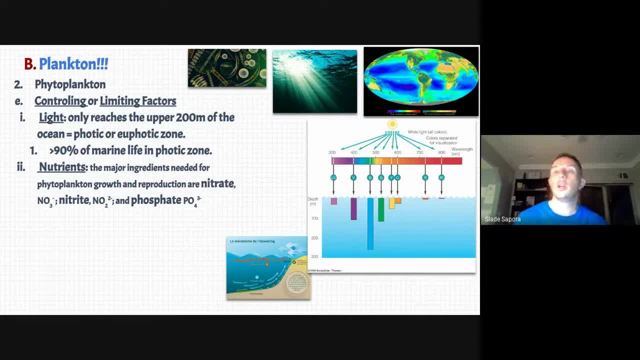 continents and they sort of pepper the ocean waters near shore and then currents will carry them further out. If you're in a shallow ocean or where two plates may converge and there's this thing called upwelling- we'll talk about that later- that can mix nutrients up. So along the 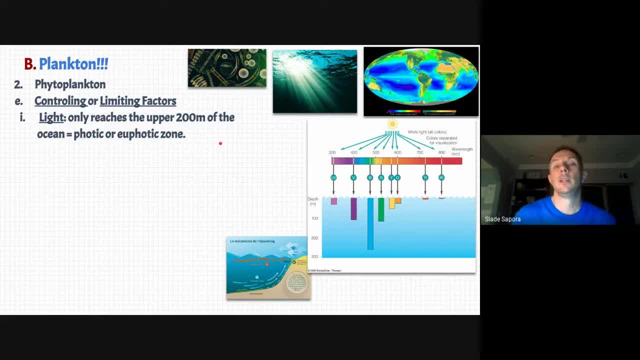 plankton. where we do is light right. so if you're doing photosynthesis, you need the photo part to do the synthesis. okay, so light only reaches the upper 200 meters of the ocean in the photic zone. below that 200 meter depth, it's 99 of all. light is gone. it's what we call the. 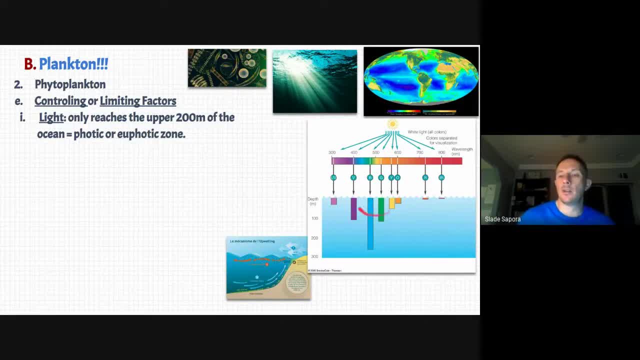 photic zone and so light doesn't penetrate, and this graphic here kind of shows what types of light and penetrate and to what depth. right, a red light is, uh penetrates the shallowest, only about 10 meters, 30 feet and it's gone. but your blue light, uh tends to penetrate the deepest, that's. 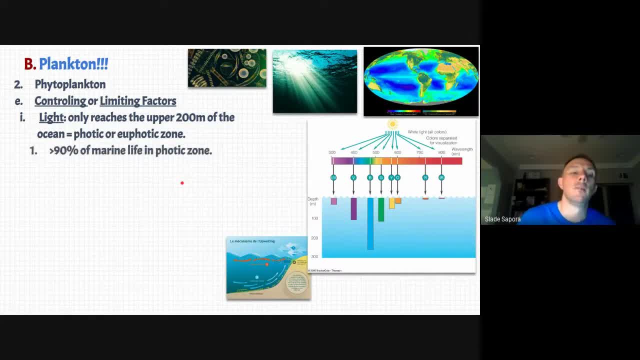 why we see the ocean is blue. coincidentally, um 90 of all marine life is in this upper 200 meters. then this up in here is the photic zone. this is where photosynthesis is happening. below this, no photosynthesis, so not much life at all. 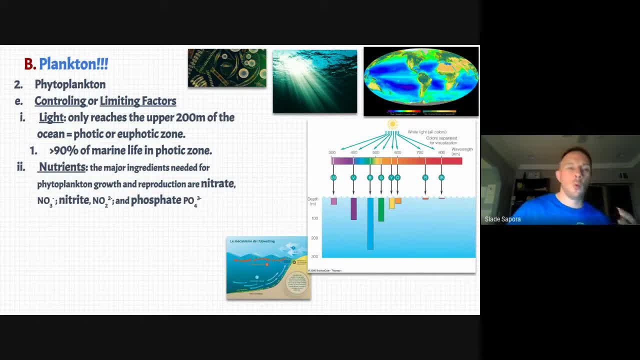 and the second thing that controls or limits where phytoplankton can occur or does occur in abundance is nutrients right. so you've got light penetrating the surface of the ocean in the upper area, but then those nutrients right, the major ingredients that these things need to produce. 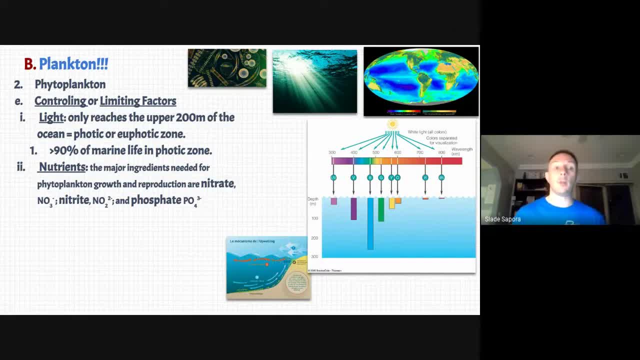 their cells and produce their bodies and make more dna and blah, blah, blah are nitrates, right nitrogen, and then phosphates as well, and these things derive and come from land and rock and rivers. right, rivers carry these things out, the wind blows them off of continents and they sort of pepper the. 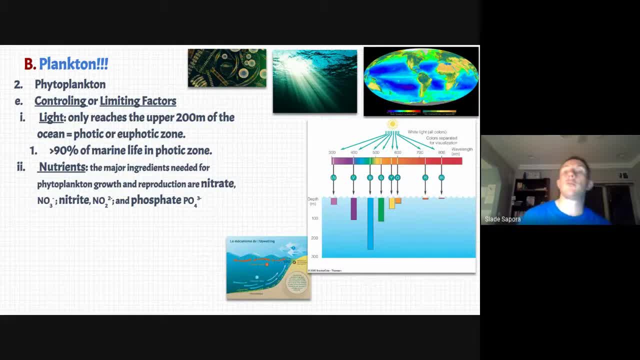 ocean waters near shore and then currents will carry them further out. if you're in a shallow ocean or where two plates may converge and there's this thing called upwelling- we'll talk about that later- that can mix nutrients up. so along the margins of continents, where it goes from very deep to 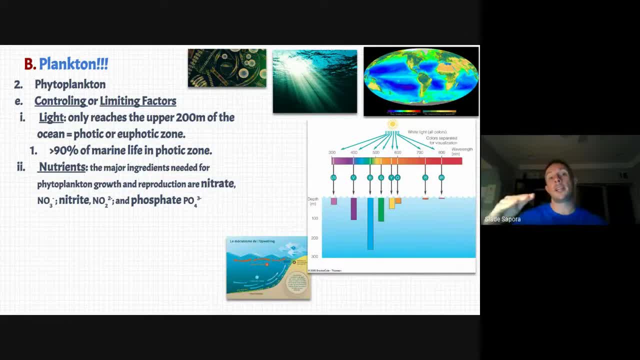 relatively shallow pretty quickly. that's where the nutrients are going to be, and then you're going to see the ocean currents will hit that shelf and then bring up all these nutrients into that photic zone. so if you've got nutrients mixing in the photic zone, oh, here i have an upwelling graphic. 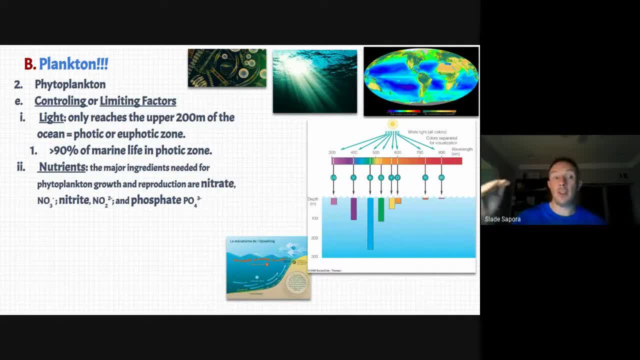 margins of continents, where it goes from very deep to relatively shallow pretty quickly. the ocean currents will hit that shelf and then bring up all these nutrients into that photic zone. So if you've got nutrients mixing in the photic zone, oh here I have an upwelling graphic right here. 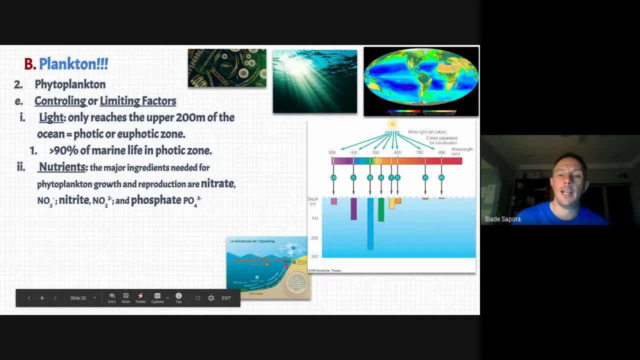 This is a perfect combination for productivity And this upwelling zone off of our particular coastline. it's about 100 miles out offshore, And so right in there you're going to get a lot of nutrients, And so if you've got nutrients mixing in the photic zone, you're going to get. a lot of nutrients mixing in the photic zone, And so, right in there, you're going to get a lot of nutrients mixing in the photic zone, And so, right in there, you're going to get a lot of nutrients mixing in the photic zone, And so, right in there, you're going to get a lot of. 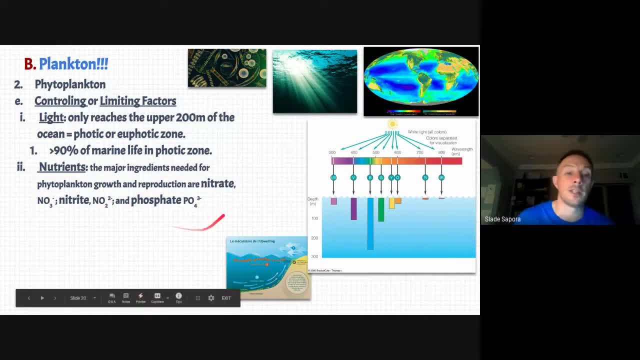 sea life and marine life, And this is where a lot of people go out to fish as well, because that's where a ton of stuff is going on. Okay, source for these nutrients is mainly run off from land And, yeah, these nutrients are used up in this upper 200 meters, So, as they're carried away, 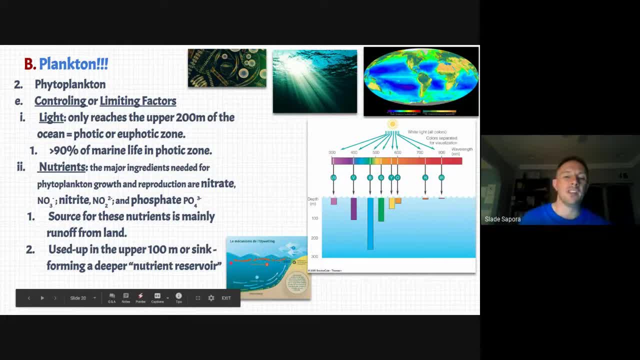 from land. as you can kind of see in this graphic here. they get used up in photosynthesis, And the farther out we get right, the more used up they get, And so eventually they're either consumed or they end up just settling and sinking down below the photic zone. 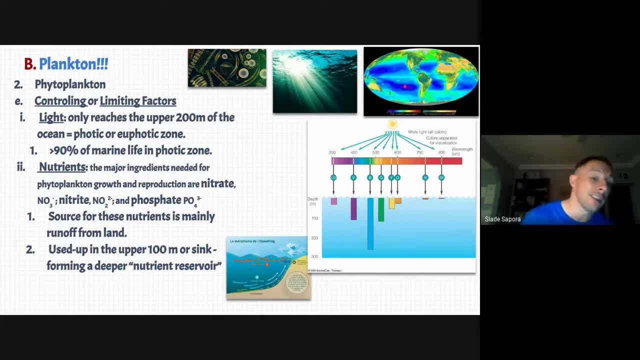 So you know, 12,000 feet deep. there's actually quite a bit of nutrients down in there, But now no sunlight so nothing can use those nutrients to grow. It's like having a bag of fertilizer in your basement. There's that map, nice and big, Okay. so yeah, you can see along the 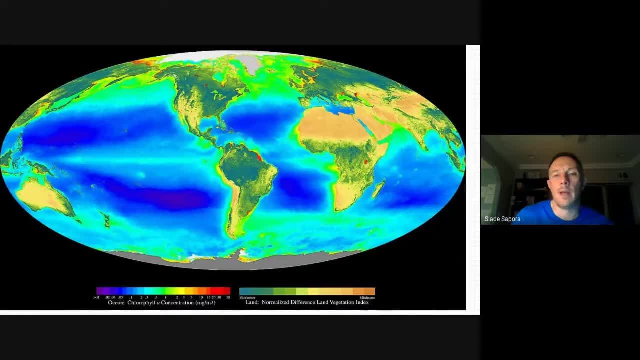 margins of continents, a lot of photosynthesis. the mouth of the Amazon River right here, you know, mouth of major rivers, mouth of Mississippi right in here, are going to be really productive areas as well. And then, yeah, I'm going to keep moving here so we can get through. 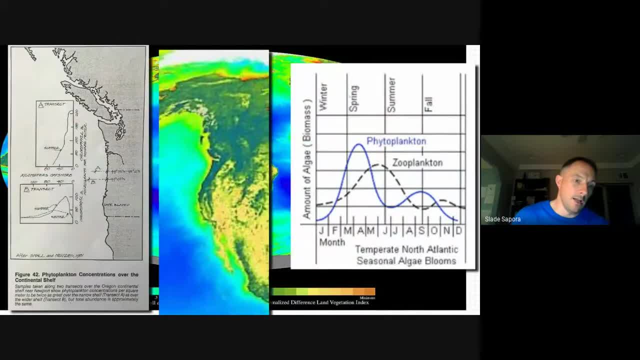 this. Okay, I'm not really going to explain these graphics too much right now, Mainly this one. here I'll take a look at The production of phytoplankton. the highest time of productivity would be in the spring. as sunlight increases, Phytoplankton production starts to increase as well, and then really. 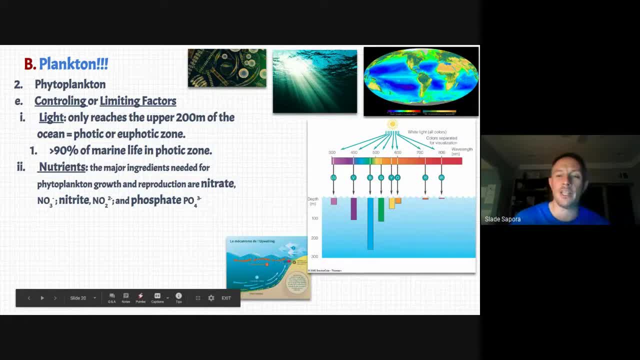 right here, um, this is a perfect combination for productivity and this upwelling zone off of our particular coastline. it's about 100 miles out offshore, and so right in there you're going to get a lot of sea life and marine life, and this is where a lot of people go out to fish as well. 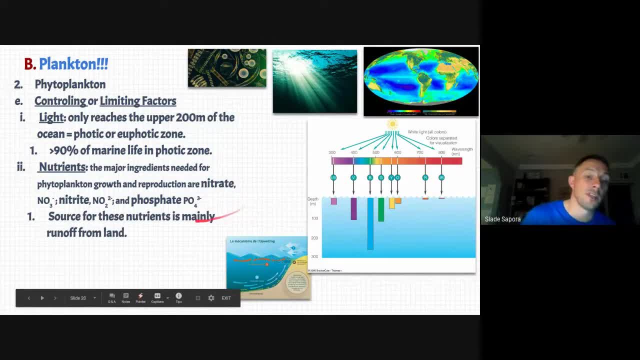 because that's where a ton of stuff is going on. okay, source for these nutrients is mainly run off from land and, um, yeah, these nutrients are used up in this upper 200 meters. so as they're carried away from land, as you can kind of see in this graphic here, um, they get used up in photosynthesis and the 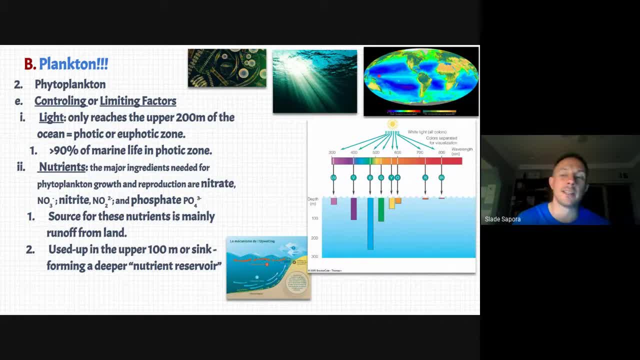 farther out we get right and the more used up they get, and so eventually, um, they're either consumed or they end up just settling and sinking down below the photo zone, so you know 12 000 feet deep. there's actually quite a bit of nutrients down in there, um. but now. 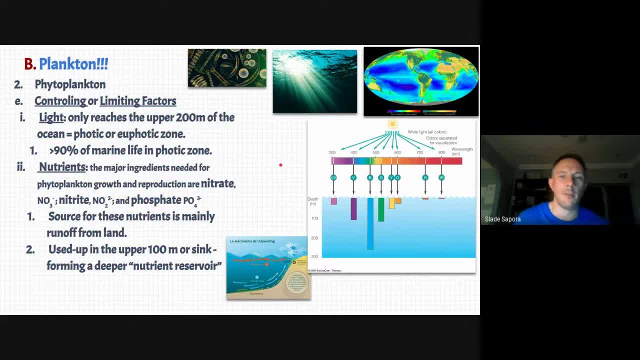 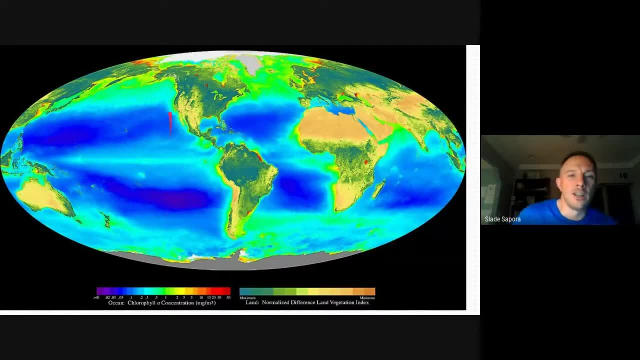 no sunlight so nothing can use those nutrients to grow. it's like having a bag of fertilizer in your basement. there's that map, nice and big, okay, so uh, yeah, you can see along the margins of continents, a lot of photosynthesis um the mouth of the amazon river, right here, you know. 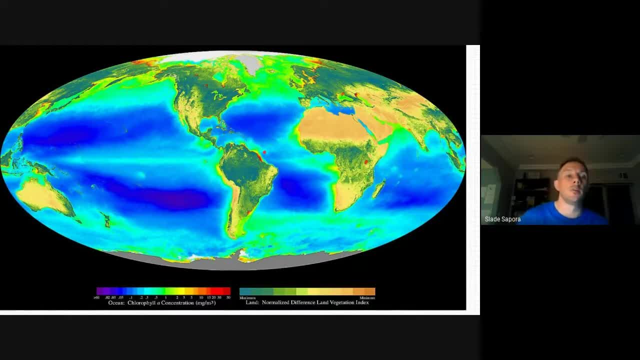 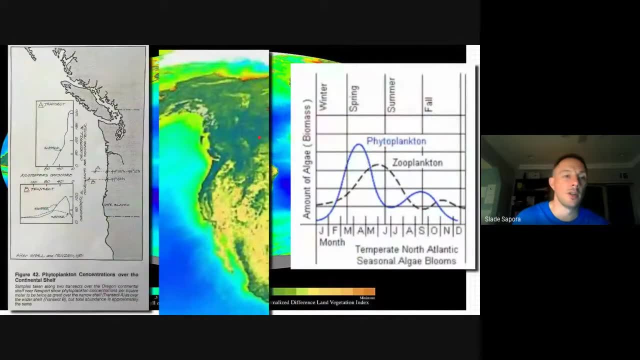 mouths of major rivers, mouth of mississippi, right in here, are going to be really productive areas as well, and then, yeah, i'm going to keep moving here so we can get through this, okay, um, yeah, i'm not really going to explain these graphics too much right now. 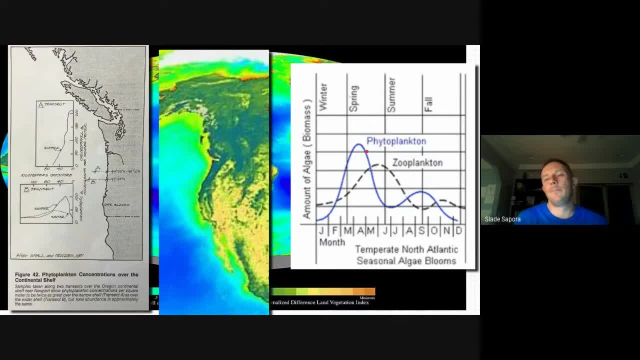 mainly this one here. i'll take a look at um the production of phytoplankton. uh, the highest time of productivity would be in the mid to late 20th century, so that's what we're talking about here. so you know, in the spring, as sunlight increases, um phytoplankton production starts to increase as. 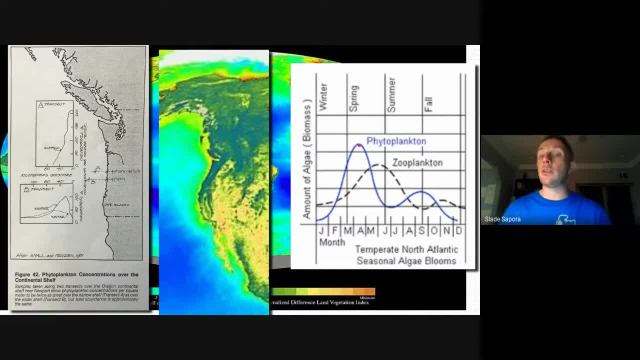 well, and then really starts to peak. you know right about now, actually out in the ocean, where we're in april here, um. but zooplankton isn't a curve that sits right on top of that. right, because it responds to that. so the phytoplankton peaks and then, as it is increasing, the zooplankton's feeding on it and 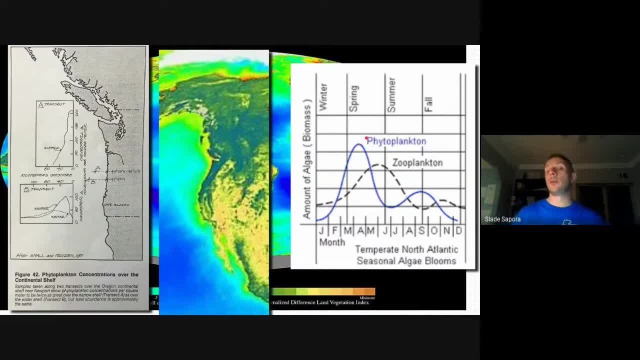 starts to peak. you know, right about now, actually out in the ocean, where we're in April here- But zooplankton isn't a curve that sits right on top of that. right, because it responds to that. So the phytoplankton peaks and then, as it is increasing, the zooplankton is feeding on it. 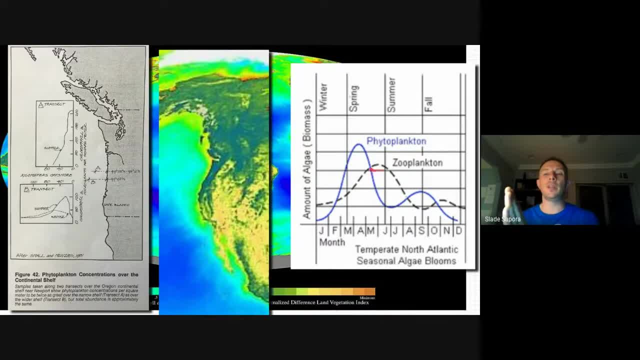 and reproducing. but they're peaking. So the phytoplankton is feeding on it and they're feeding on it. So the phytoplankton peak is a little bit after that peak of the phytoplankton as well. 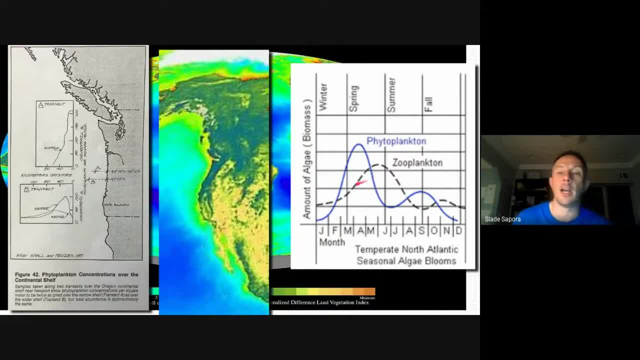 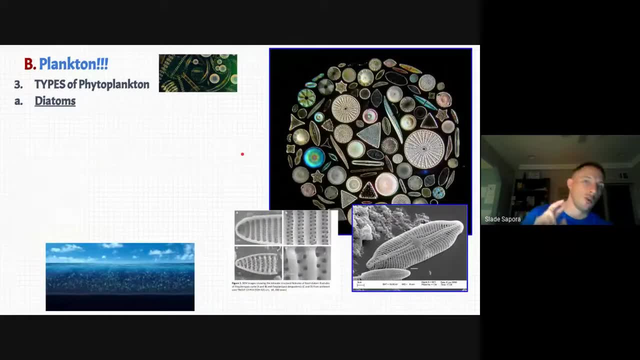 more in June. That's when you'd see the highest numbers of zooplankton in the oceans. Okay, Types of phytoplankton. We're almost done here. Two types of phytoplankton that I want you to know about, the most abundant ones in the ocean. The first ones are diatoms. These are actual images. 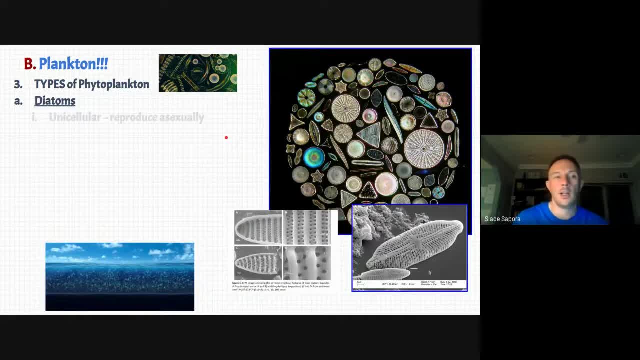 of diatoms. They are incredible looking. They are unicellular, Meaning they're single-celled, And they reproduce asexually. There is some forms of sexual reproduction here with these guys that help increase genetic variations, But the main thing is genetic diversity. The main thing is that they can reproduce asexually so they can respond. 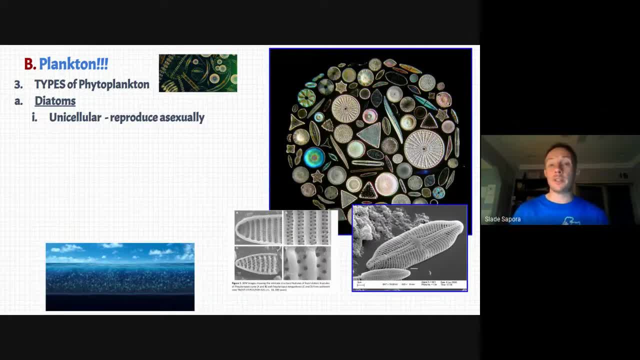 really rapidly to increases in light or food or nutrients and things like that, And their numbers can grow quickly. They're incredibly tiny, right? So they're 50 to 500 micrometers. Again, if we had microscopes we could zoom in on these. 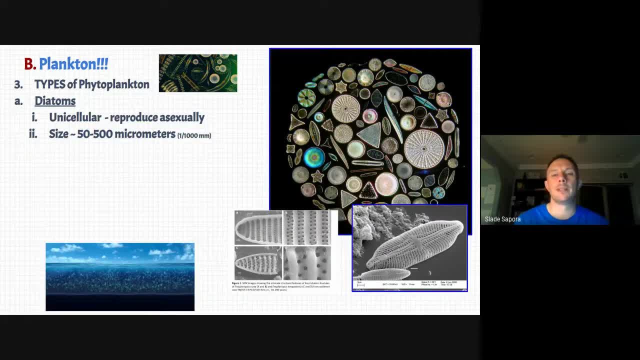 things and take a look, But basically you can fit 1,000 micrometers on a single millimeter. So if you look at a ruler and see how big a millimeter is, picture fitting 1,000 micrometers across there. All right, And just like plants, they contain chloroplasts, which are the things that do. 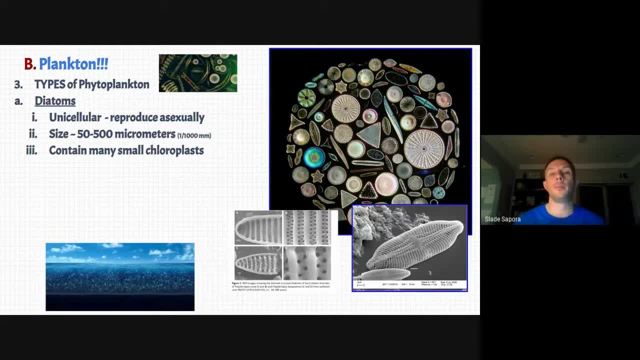 photosynthesis Plants on land evolved from these things in the ocean right, These diatoms, and then algaes that came later. The cell wall of a diatom is called a frustule- It's just a weird sounding word- And it's made of silica, It's made of quartz, It's made of glass, basically, And because it's 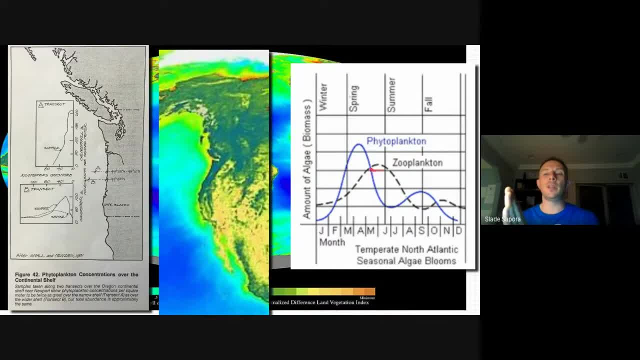 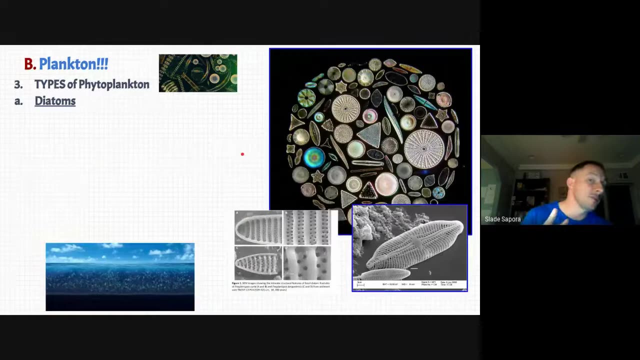 reproducing, but their peak is a little bit after that peak of the phytoplankton as well. more in um june. that's when you see the highest numbers of zooplankton in the oceans. okay, types of phytoplankton. we're almost done here. two types of phytoplankton that i want. 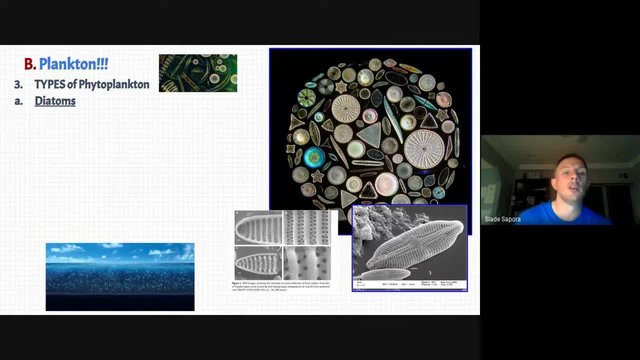 uh you to know about the most abundant ones in the ocean. the first ones are diatoms. these are actual images of diatoms. they are incredible looking. uh, they are unicellular, meaning they're single-celled, and they reproduce asexually. there is some forms of sexual reproduction here, with 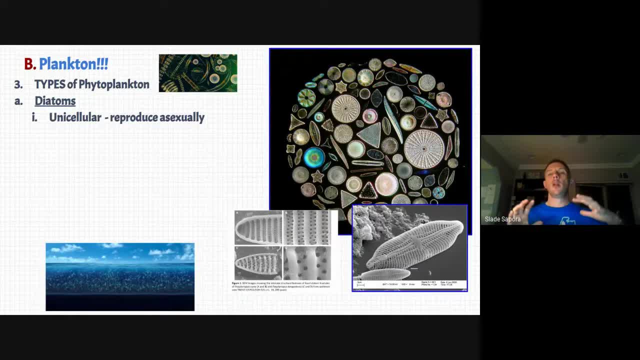 guys that help increase genetic variations, but the main thing is genetic diversity. the main thing is, um that they can reproduce asexually, so they can respond really rapidly to increases in light or food or nutrients and things like that, and their numbers can grow quickly. um, they're incredibly tiny, right, so they're um 50 to 500 micrometers again if we had microscopes. 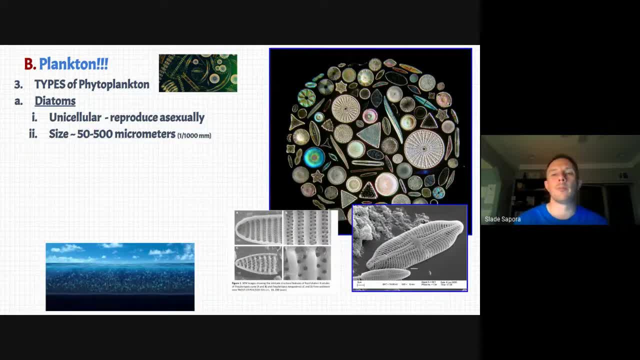 we could zoom in on these things and take a look, um, but basically you can fit 1 000 micrometers on a single millimeter. so if you look at a ruler and see how big a millimeter is, picture fitting a thousand micrometers across there. um, all right. and just like plants, they contain chloroplasts. 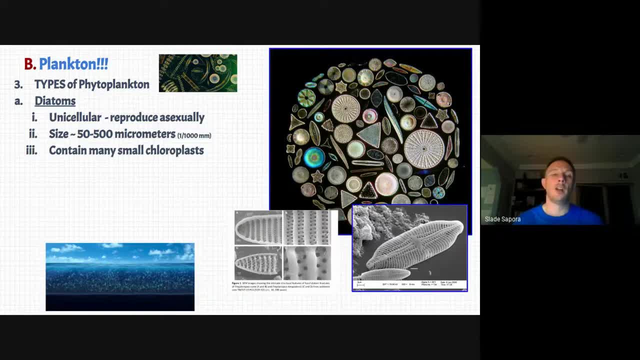 which are the things that do photosynthesis. plants on land evolved from these things in the ocean, diatoms, and then algaes that came later. The cell wall of a diatom is called a frustule- It's just a weird sounding word, And it's made of silica, It's made of quartz, It's made of. 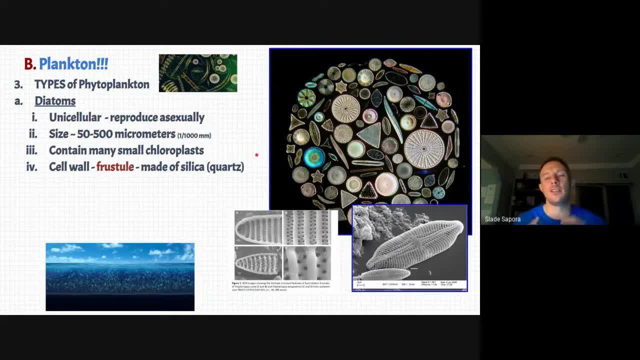 glass basically, And because it's made of quartz and glass. you know, this is their little effort to not be eaten. basically It's their defense. Because it's made of glass, they fossilize really well And they have these really cool patterns that you can see. 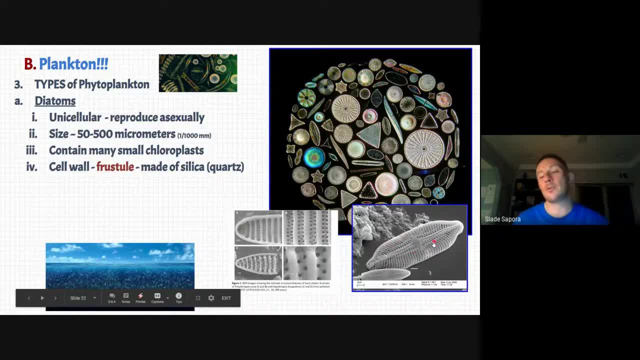 under microscopes, And each one, each species or each group, has a unique set of characteristics and patterns, And there's just an abundance of them out there in the world, And we can look back in the fossil record as well and find these throughout marine layers that go back. 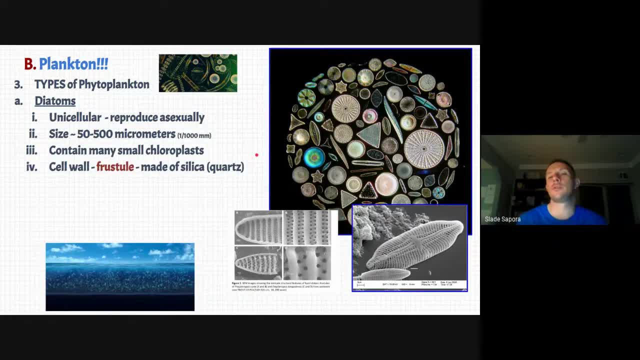 made of quartz and glass. you know, this is their little effort to not be eaten. basically It's their defense, Because it's made of glass. they fossilize, They fossilize really well And they have these really cool patterns that you can see under. 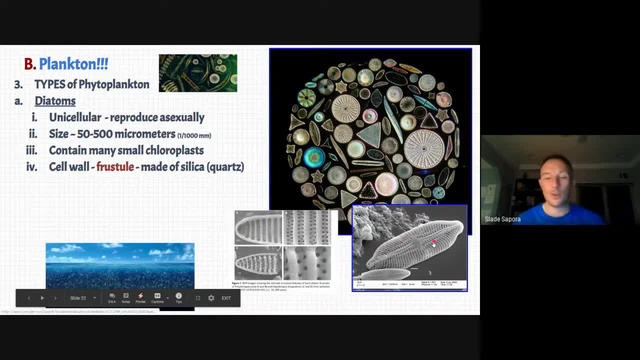 microscopes, And each one, each species or each group, has a unique set of characteristics and patterns, And there's just an abundance of them out there in the world, And we can look back in the fossil record as well and find these throughout marine layers that go back hundreds of millions of. 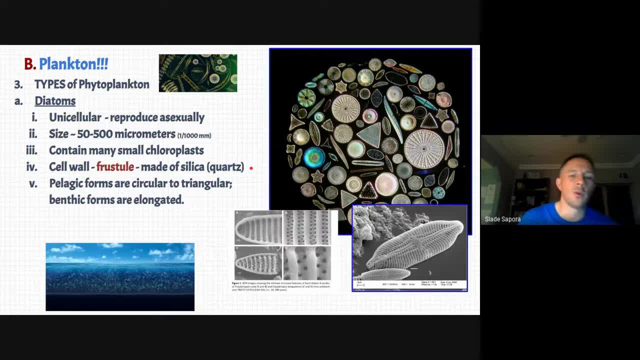 years. Okay, Pelagic forms, meaning ones that are kind of free-floating planktonic in the ocean. those tend to be more circular or triangular. And then benthic forms. By benthic we mean existing on the bottom, So these would be in. 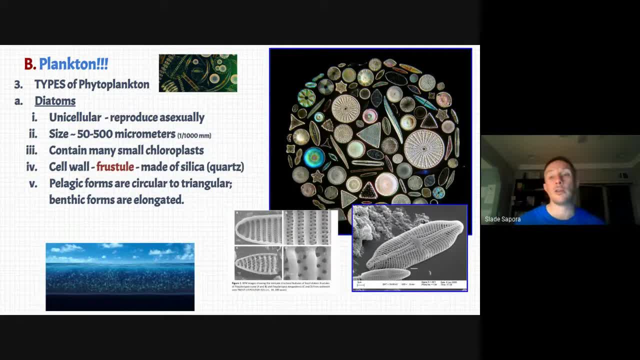 shallow waters, where light touches the bottom bays, estuaries near shore. Those ones tend to be more linear and elongated And they kind of spike themselves into the mud and kind of stick up and gather sunlight. It's like a microscopic garden of grass that you can't really see, which is kind of. 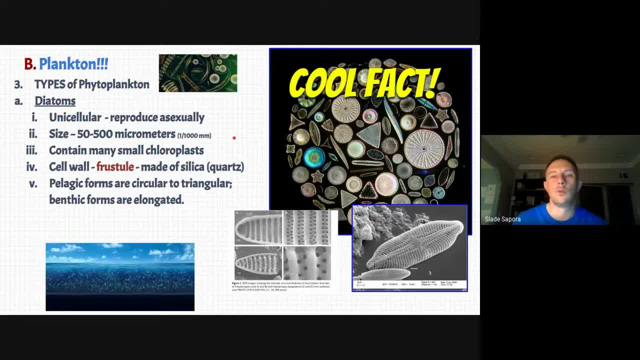 cool to think about. that's out there. Cool fact: There are 100 micrometers in a millimeter. I don't know why I put that there, because there are 1,000 anyway. You know I make this presentation late and it is late, So whatevs? Yeah, All right, I need. 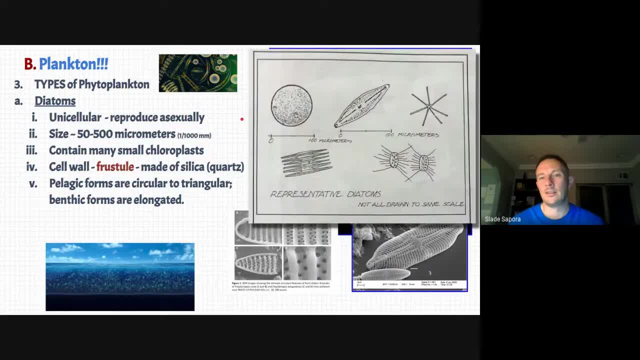 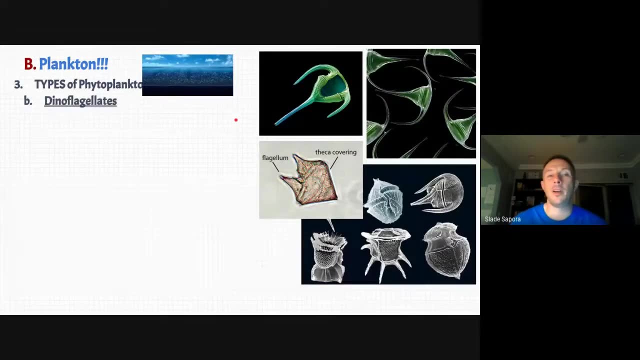 to go and fix that. Uh-huh, There we go, So you can kind of see the size of these things as well in relation here On the micrometer scale. Okay, The other type of phytoplankton we're going to talk about are: 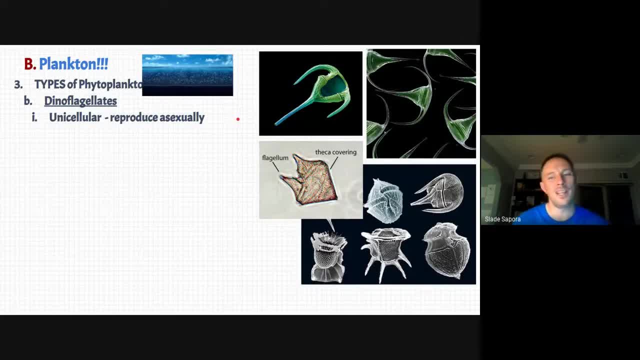 dinoflagellates. They also are unicellular, meaning they're single-celled. They're called dinoflagellates- The di refers to the two part and then flagella, So these are kind of like little whips that they can move with through the water. It's kind of cool. Actually. they tend to. 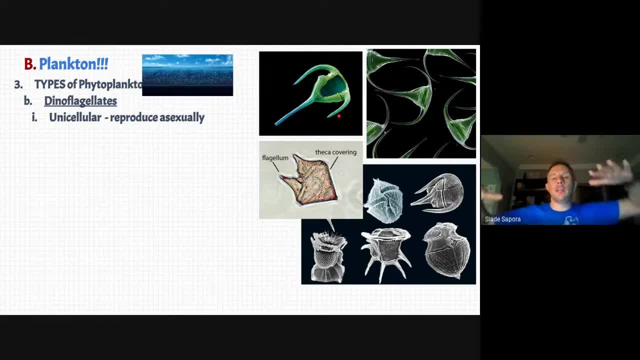 move with the rear one and the two on top kind of give them blisters, So they're kind of like a buoyancy to keep them from sinking, which is kind of cool to think about. It kind of spreads out the surface area and lets them float. They also reproduce asexually, and again very tiny as well. 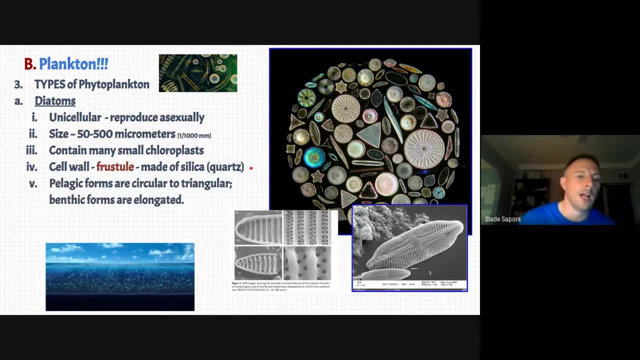 hundreds of millions of years. Okay, Pelagic forms, meaning ones that are kind of free-floating planktonic in the ocean. Those tend to be more circular or triangular, And then benthic forms. By benthic we mean 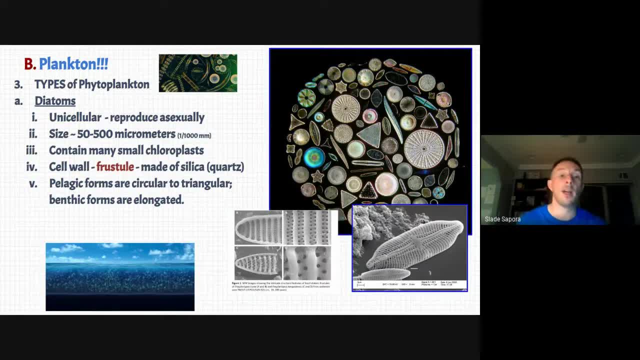 We mean existing on the bottom, So these would be in shallow waters where light touches the bottom, bays, estuaries, near shore. Those ones tend to be more linear and elongated And they kind of spike themselves into the mud and kind of stick up and gather sunlight. It's like a microscopic. 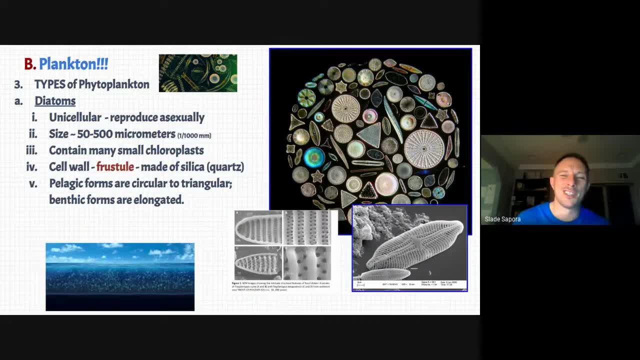 garden of grass that you can't really see, which is kind of cool to think about. that's out there. Cool fact: There are 100 micrometers in a millimeter. I don't know why I put that there, because there are 100 micrometers in a millimeter. I don't know why I put that there, because there. 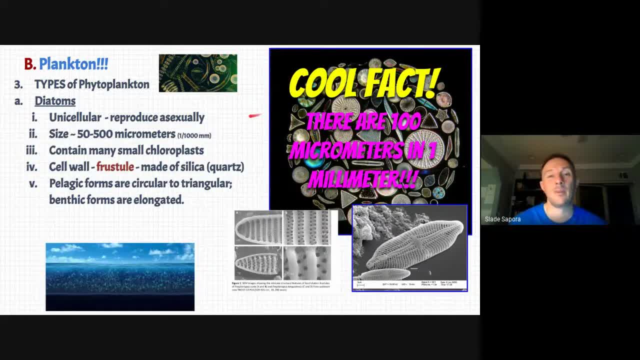 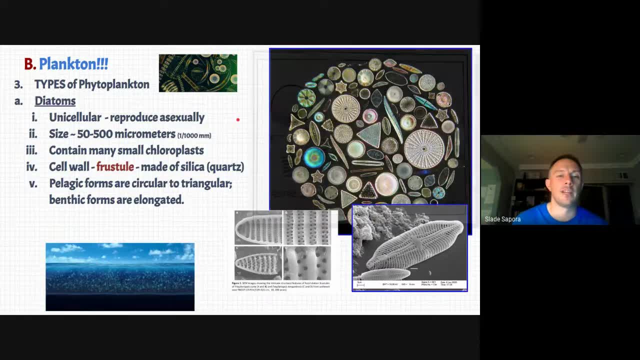 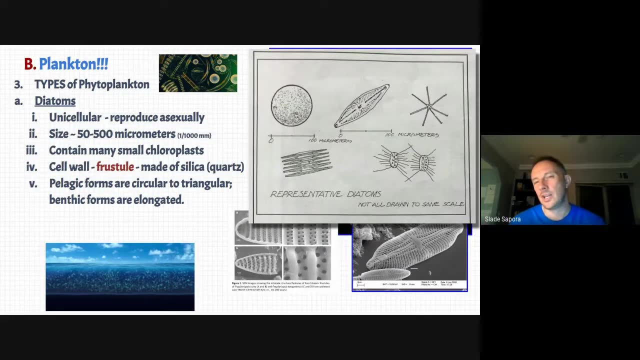 are 1,000. anyway. I make this presentation late and it is late, so whatevs? Yeah, All right, I need to go and fix that. Uh-huh, There we go, So you can kind of see the size of these things as well. 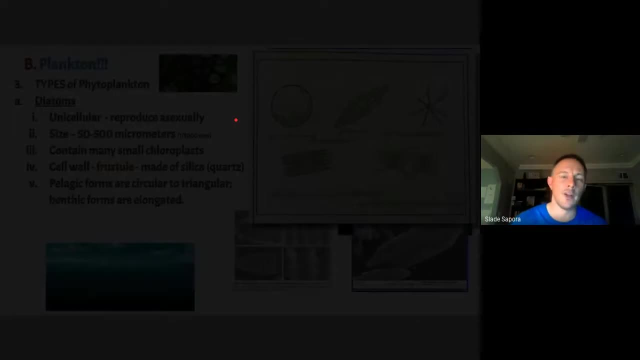 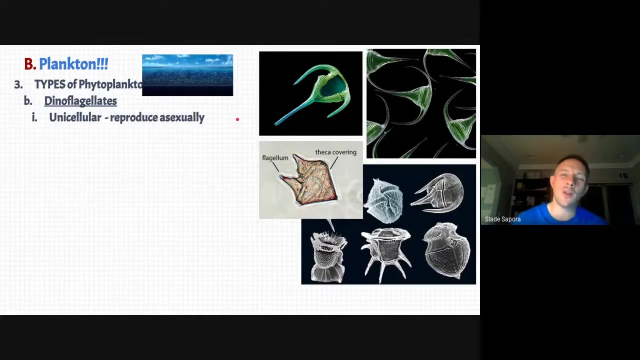 in relation here on the micrometer scale. Okay, The other type of phytoplankton we're going to talk about is phytoplankton, And I'm going to talk about phytoplankton And I'm going to talk about are dinoflagellates. They also are unicellular, meaning they're single-celled. They're called 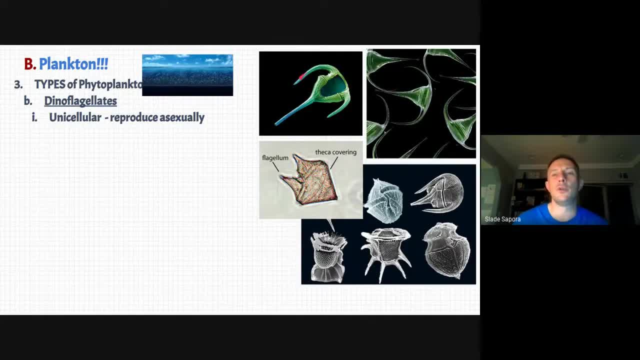 dinoflagellates. The di refers to the two part and then flagella, So these are kind of like little whips that they can move with through the water. It's kind of cool. Actually, they tend to move with the rear one and the two on top kind of give them buoyancy to keep them from sinking. 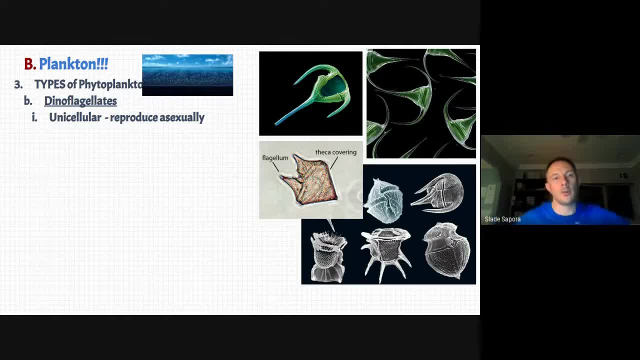 which is kind of cool to think about. It kind of spreads out the surface area and lets them float. They also reproduce, And again very tiny as well: 25 to 1,000 micrometers in size, Two you know they can be. 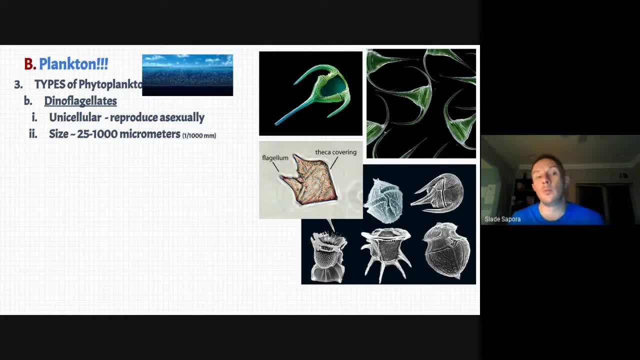 25 to 1,000 micrometers in size Two, you know they can be large. They have the two flagella for movement and again for flotation as well, And the cell wall of these guys is made of cellulose, so not the silica that you'd see in the diatoms. 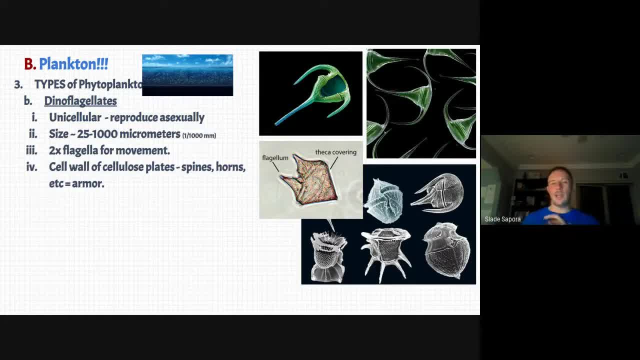 And the cell wall is kind of rougher on these. It isn't quite as ornate or polished, but they have these little spikes and horns And again it's a form of armor to try and keep them from being eaten. They contain many small chloroplasts, just like the diatoms. Plants do as well. 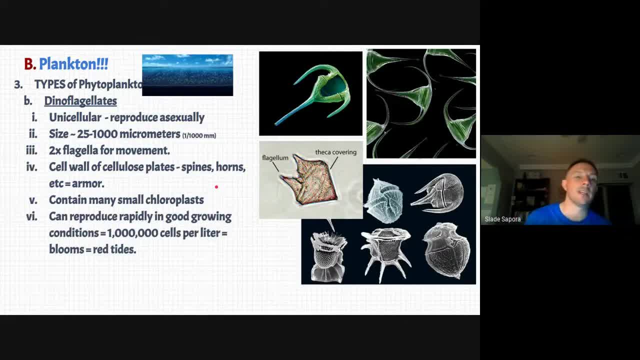 allow them to do photosynthesis, And because they reproduce asexually, they can reproduce really rapidly in good growing conditions. So here this time of year- right now, it's starting to be peak time for plankton- Days are getting longer, Weather's getting nicer, And they're responding to that rapidly. So 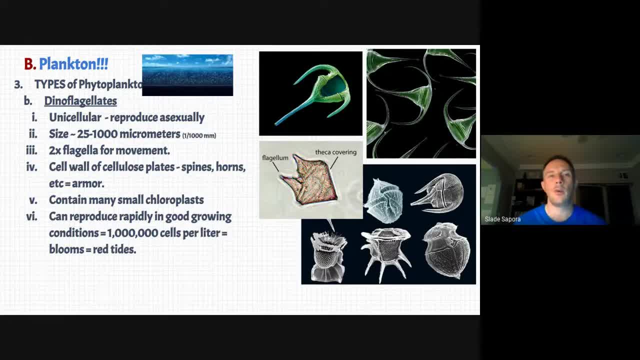 where in the wintertime you could go out and go scuba diving here and you could see, you know, 30,, 40,, 50, 60 feet, maybe in the water, underwater, with a mask on. It'd be that clear. 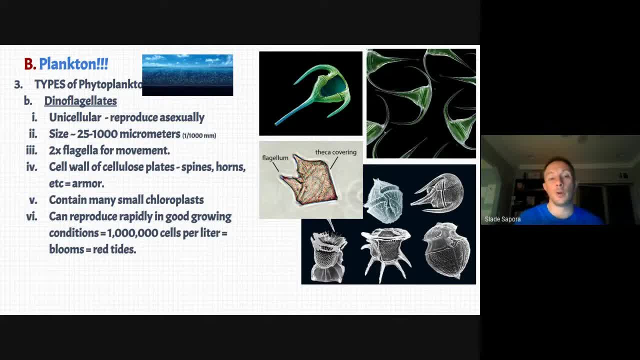 You know there may be- just you know- 10 or 20 of these guys per liter of water. A liter of water is like an algae bottle, But ramp up to now. in about April, the water gets so cloudy you can barely see your hand out in front of your face, And that's because there's more than 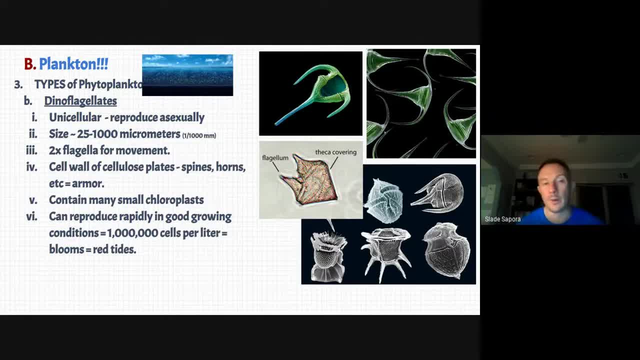 one million of these per liter of water And they, you know they, reproduce really fast and rapidly. They call them blooms, because they'll go from you know one to a million in a matter of per liter, in a matter of you know a month or so, And they often give the water this sort of red. 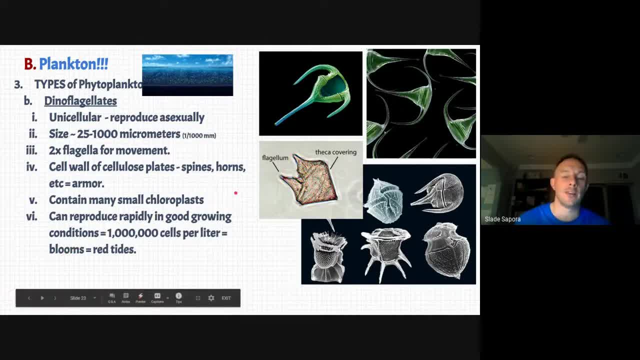 burgundy color and they call it red tide. as a result of that, There gets to be so many in the water. They produce toxins as a waste product. Demoic acid is one of the byproducts that they produce just through their general metabolism. It's not a problem when there's only a few in the water. 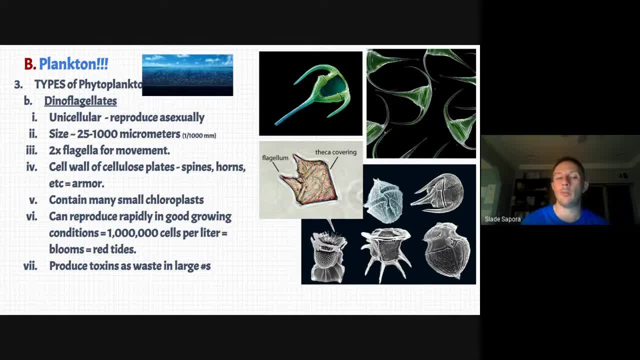 but when there's a million per liter in the water it does become a problem. That demoic acid that they're kind of giving off as like a waste product, almost like they're peeing it out, gets really concentrated in the ocean water And then things that are filter feeders in the ocean. 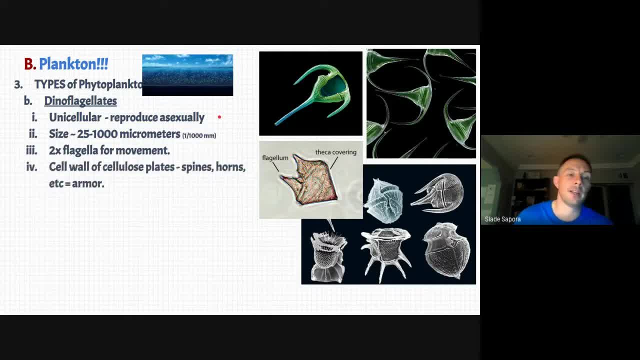 large. They have the two flagella for movement and again for flotation as well, And the cell wall of these guys is made of cellulose, So not the silica that you'd see in the diatoms, And the cell wall is kind of rougher on these. It isn't quite as ornate or polished, but they have these little. 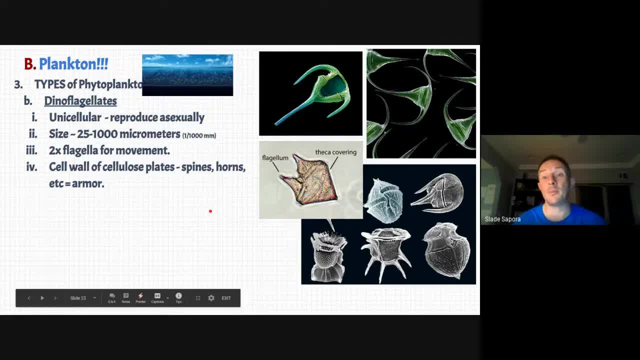 spikes and horns And the cell wall is kind of rougher on these. It isn't quite as ornate or polished, but they have these little spikes and horns And the cell wall is kind of rougher on these And again it's a form of armor to try and keep them from being eaten. They contain many small. 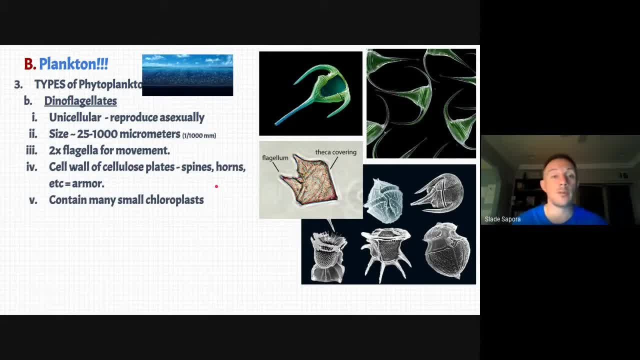 chloroplasts, just like the diatoms Plants do as well, Allow them to do photosynthesis, And because they reproduce asexually, they can reproduce really rapidly in good growing conditions. So here this time of year, right now, it's starting to be peak time for plankton. 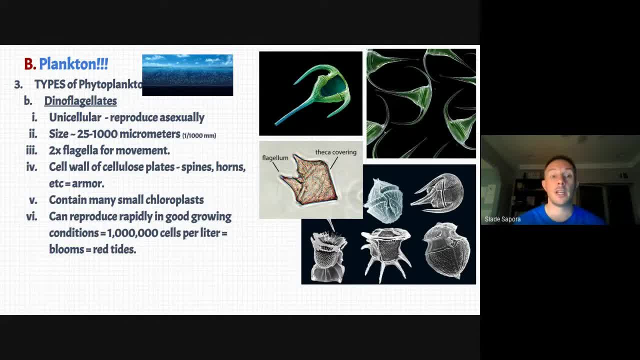 Days are getting longer, Weather's getting nicer And they're responding to that rapidly. So where in the wintertime you could go out and go scuba diving here and you could see 30,, 40,, 50,, 60 feet maybe in the water underwater. with a mask on, It'd be that clear. There may be just 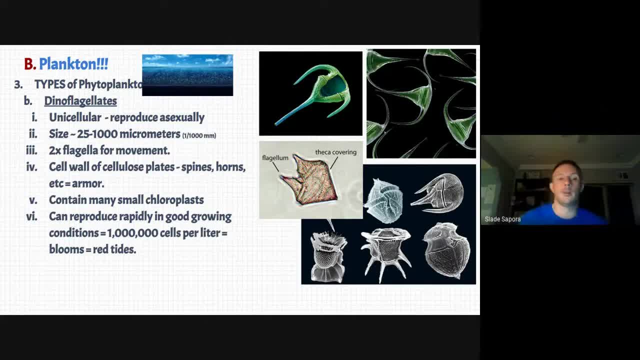 10 or 20 of these guys per liter of water. A liter of water is like an algae bottle, But ramp up. to now. in about April, the water gets so cloudy you can barely see your hand out in front of your face, And that's because there's more than 1 million of these per liter. 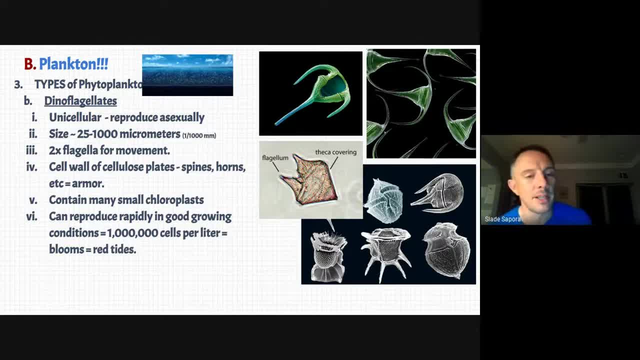 of water, And that's because there's more than 1 million of these per liter of water, And that's they reproduce really fast and rapidly. They call them blooms, because they'll go from one to a million per liter in a matter of a month or so, And they often give the water this sort of 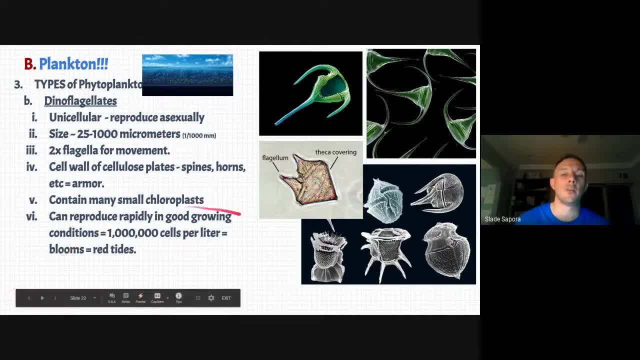 red, burgundy color and they call it red tide. As a result of that, there gets to be so many in the water. They produce toxins as a waste product. Demoic acid is one of the byproducts they produce just through their general metabolism. It's not a problem when there's. 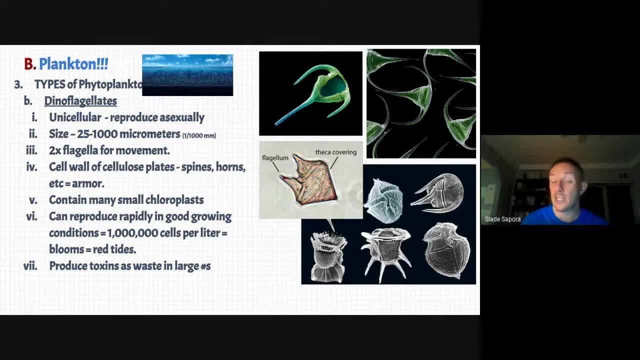 only a few in the water, but when there's a million per liter in the water it does become a problem. That domoic acid that they're kind of giving off as like a waste product, almost like they're peeing it out, gets really concentrated in the ocean water And then things that are 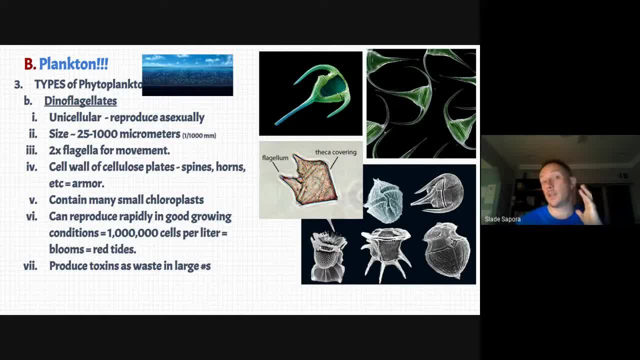 filter feeders in the ocean, such as clams or even things like crabs that pull in a lot of water through their gills, will get a buildup of this in their body tissue and they become toxic to us to eat. So that's why we have these shellfish closures like that on the Oregon coast. 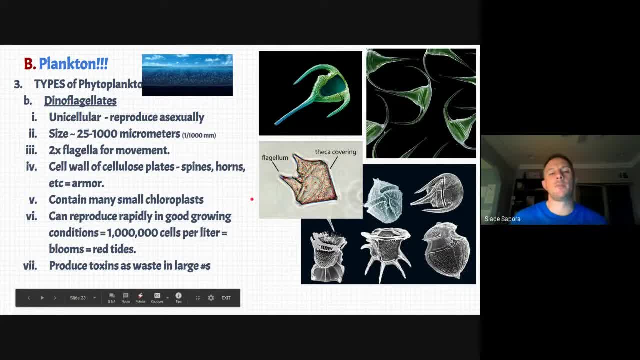 In response to that, because they got so much of this built up in them and then again it'll be able to eat them again in the winter. So usually in the summer months- spring to summer- we avoid eating things like clams and mussels on the coast. 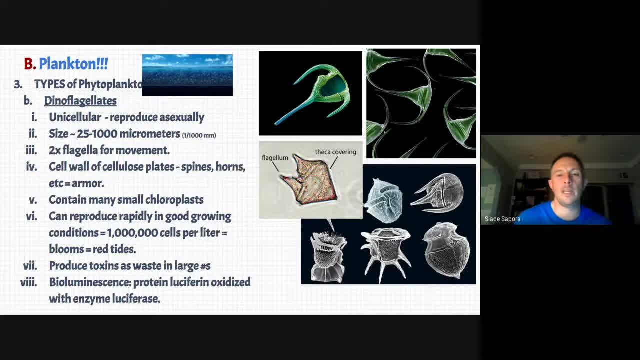 They also produce this bioluminescence, meaning that they kind of get this glowy thing at night kind of like a firefly, And they have a protein that they produce called luciferin- kind of funny- And it gets oxidized. 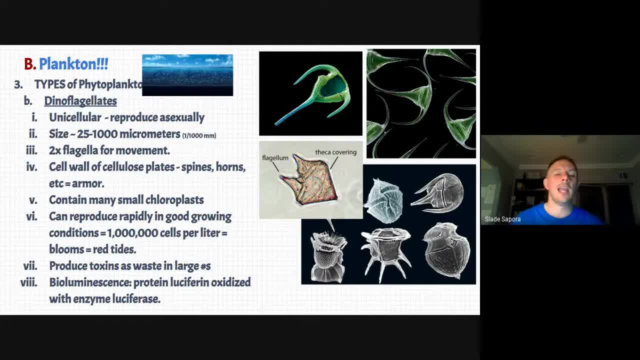 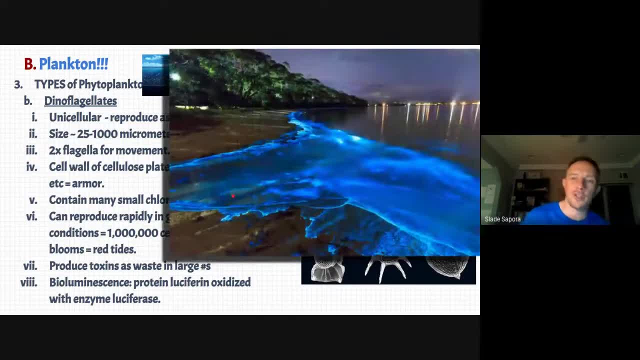 with this specific enzyme called luciferase And it lights up, it creates light, And let me see if I have a picture of that here. I sure do. So here's kind of a little bit of a time-lapsy shot of this bioluminescence. If you've ever been out on the beach at nighttime walking here, 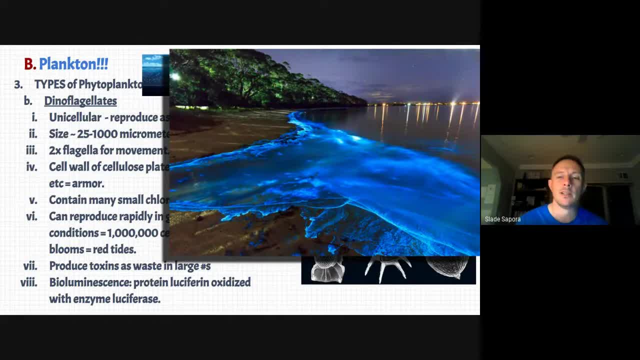 check it out. We're coming into the red tide months, So especially in May and June. sometimes you'll be able to see this if you just kind of watch the waves roll in And if you walk right as the wave is washing out, your feet kind of contacting it. 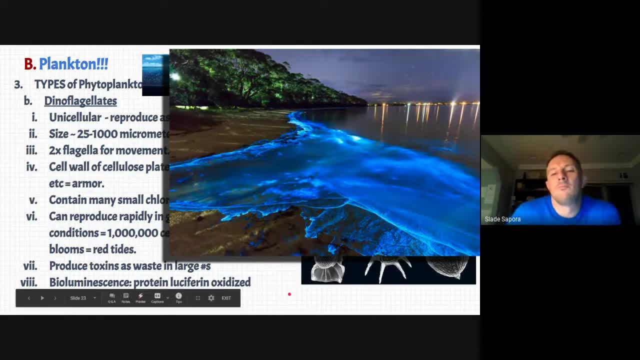 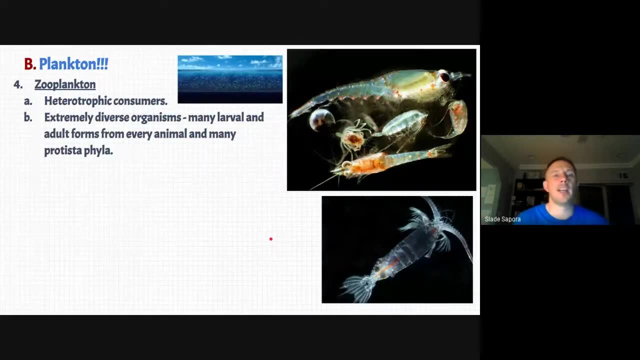 will cause it to oxidize And you'll see this light. It's kind of cool. Look at there someone's hand moving through it. Okay, Zooplankton, we got our heterotrophic consumers. These are the things that consume or eat the phytoplankton. the next level up in the 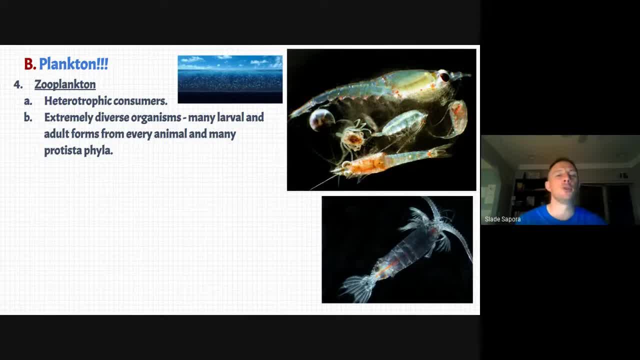 old energy pyramid food web. This is a huge group of organisms, extremely diverse. We've got larval adult forms of pretty much everything in the ocean, but really, at some point, is plankton. It seems like many things are plankton their whole lives, When we think of zooplankton. 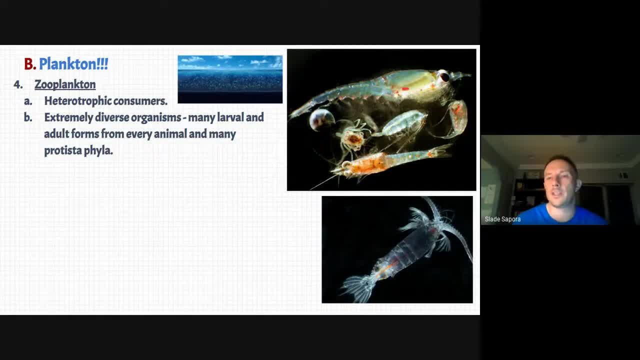 we tend to think of things like shrimp Euphazids here, or copepods with their little antennas and things like that, But they're also things like I said: larval crab, larval plants, larval worms, larval everything Okay. 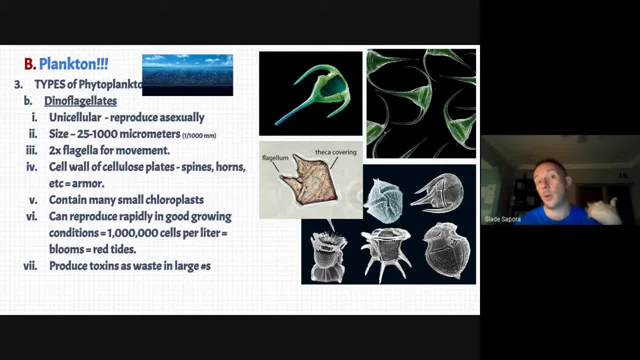 such as clams or even things like crabs that you know pull in a lot of water through their gills, will get a buildup of this in their body tissue and they become toxic to us to eat. So that's why we have these shellfish closures. 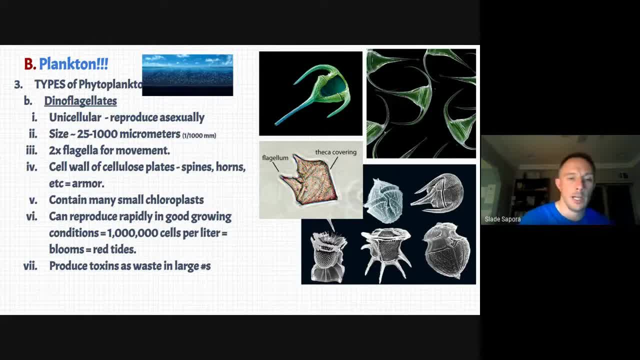 like that on the Oregon coast In response to that, because they got so much of this built up in them and then again it'll be able to eat them again in the winter. So usually in the summer months- spring to summer- we avoid eating things like clams and mussels on the coast. 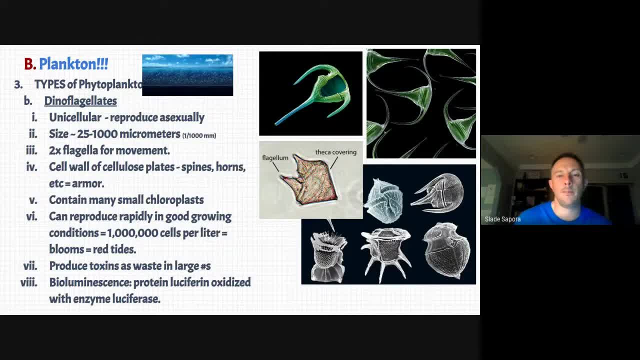 They also produce this bioluminescence, meaning that you know, they kind of get this glowy thing at night kind of like a firefly, And they have a protein that they produce called luciferin- kind of funny- And it gets oxidized. 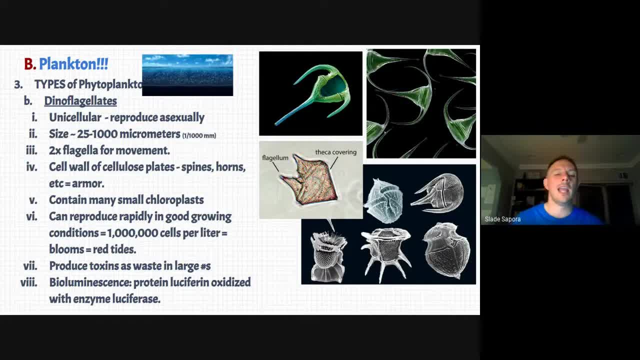 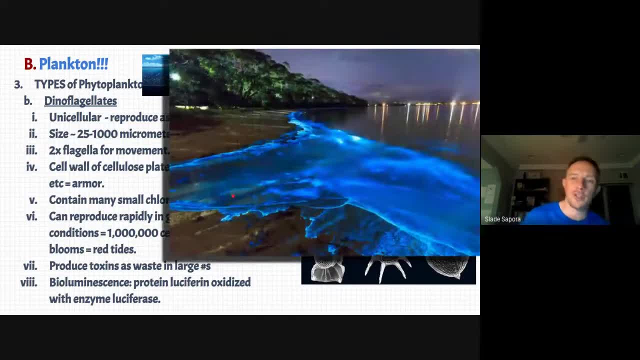 with this specific enzyme called luciferase And it lights up, it creates light, And let me see if I have a picture of that here. I sure do. So here's kind of a little bit of a time-lapse-y shot of this bioluminescence. If you've ever been out on the beach at nighttime- 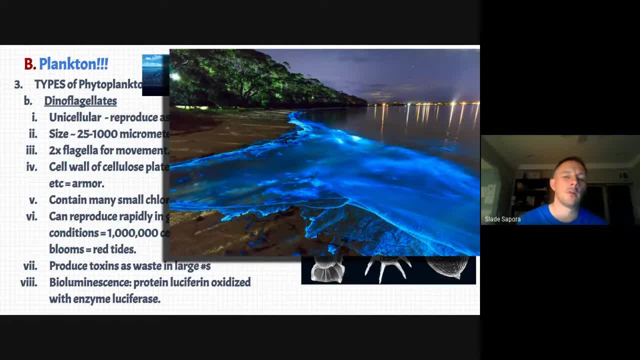 walking here check it out. We're coming into the red tide months, So especially in May and June, sometimes you'll be able to see this if you just kind of watch the waves roll in. And if you walk right as the wave is walking, washing out your feet, kind of contacting it, will cause it to. 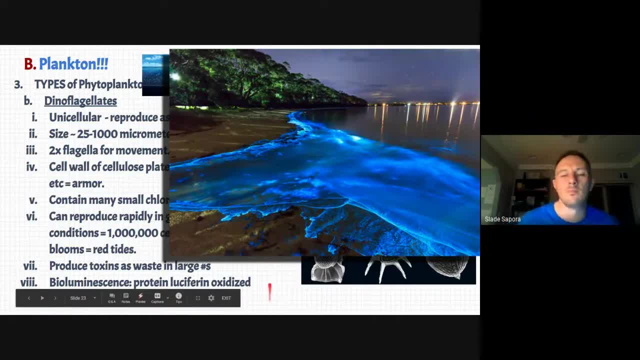 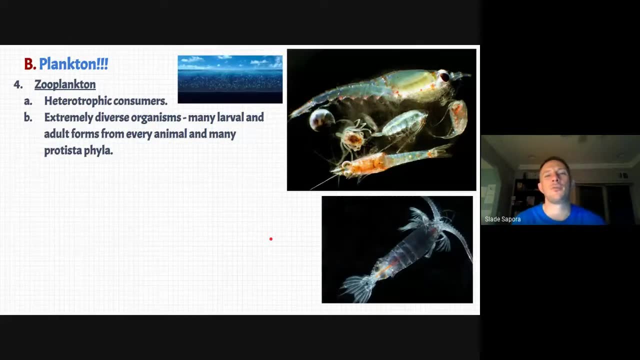 oxidize And you'll see this light. It's kind of cool. Look at that. There's someone's hand moving through it. Okay, Zooplankton, we got our heterotrophic consumers. These are the things that consume or eat the phytoplankton. 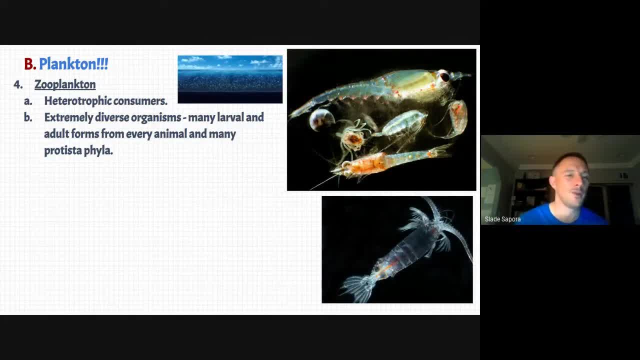 the next level up in the old energy pyramid food web. This is a huge group of organisms, extremely diverse. We've got larval adult forms of you know just pretty much everything in the ocean, but really, at some point, is plankton. 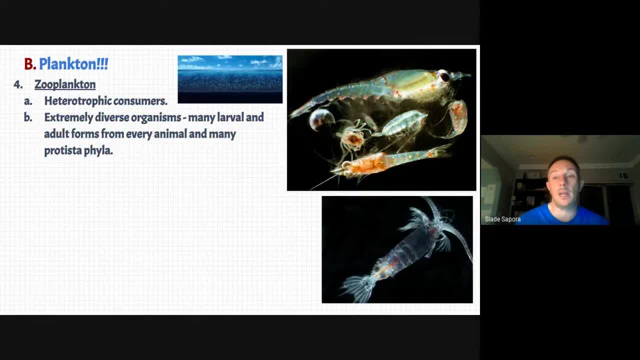 It seems like in May many things are plankton their whole lives. When we think of zooplankton we tend to think of things like shrimp euphasids here or copepods with their little antennas and things like that. But there are also things like I said. 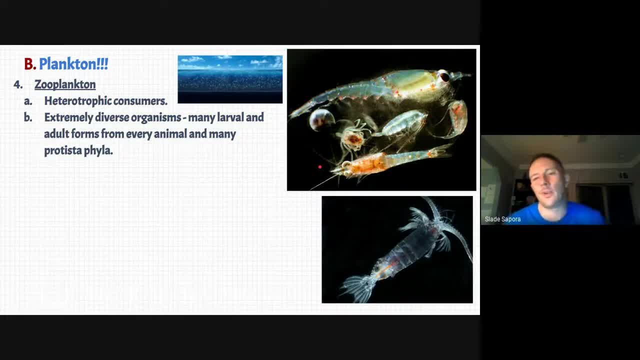 larval crab, larval plants, larval worms, larval everything. Okay, The most important group would be these copepods. Again, they're a type of a crustacean, So they're in the group arthropoda, which is the largest group of animals on the planet. 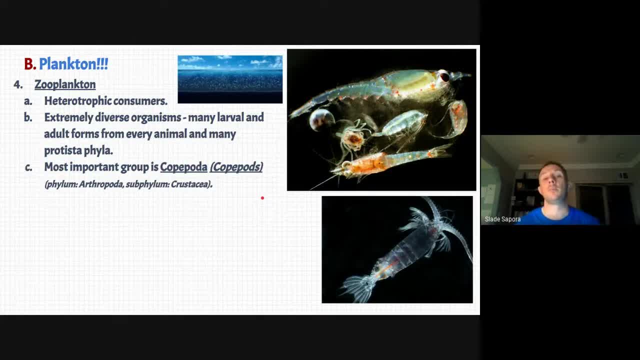 Includes insects and arachnids, millipedes, dragonflies and crustaceans, crustaceans of crabs and shrimps, and all these other things as well. It's a huge, huge, huge, diverse group. 80% of all planet animals are arthropods and a chunk of that are crustaceans. 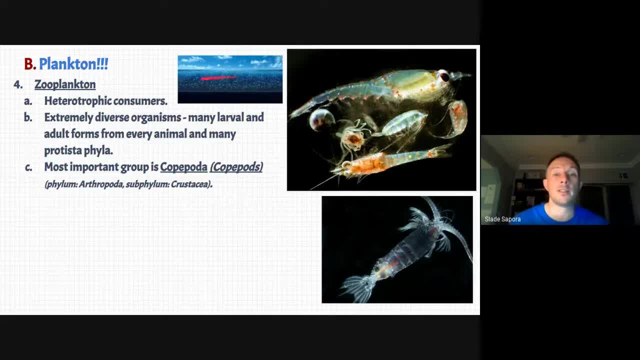 But just pure abundance, pure numbers. copepods: they're more numerous than any other type of animal on the planet. They're everywhere in the oceans because they're small, So, um, yeah, one to three millimeters in size. you can kind of see the moving in the water, but you can't really tell what it is unless you have a microscope. 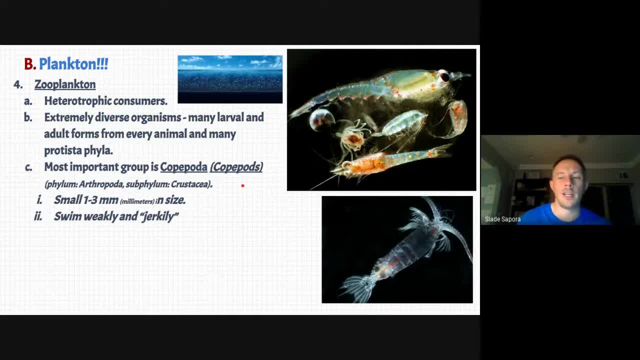 They swim weakly and jerkily. They use their little antenna to float and again to help give them buoyancy. Again, large antennas slow their state of rate of sinking. and that's the same as with dendroflagellates we were just talking about. 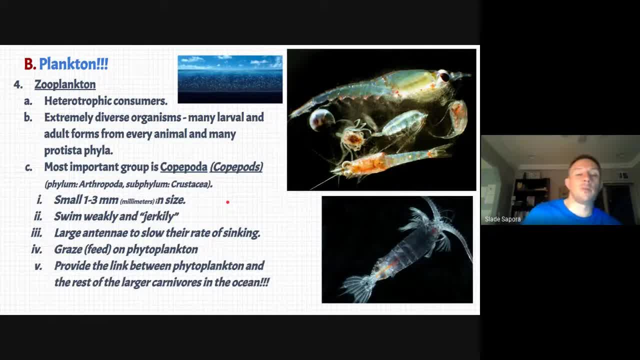 They graze and feed on phytoplankton And they provide a link between that phytoplankton and the larger carnivores. So things that eat the copepods maybe don't necessarily eat the phytoplankton. So if really the copepods weren't there, pretty much life in the ocean would kind of stop. 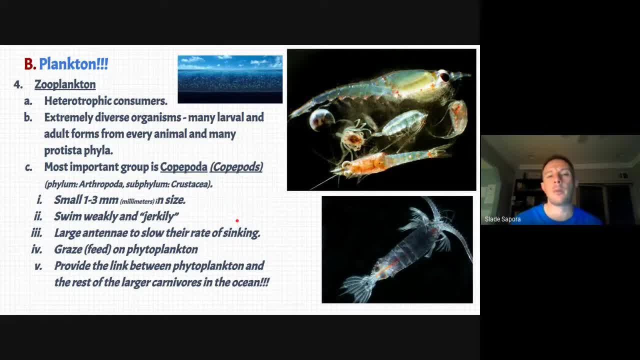 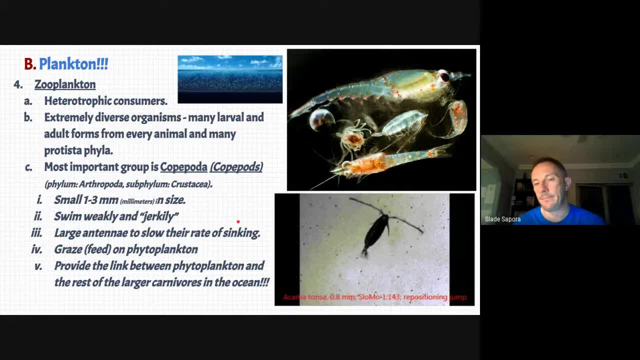 They are that link between those super, you know, microscopic phytoplankton and other things as well. Here's a picture of one moving jerkily through the water using their antenna. Okay, wonderful. Oh look, there's another one. 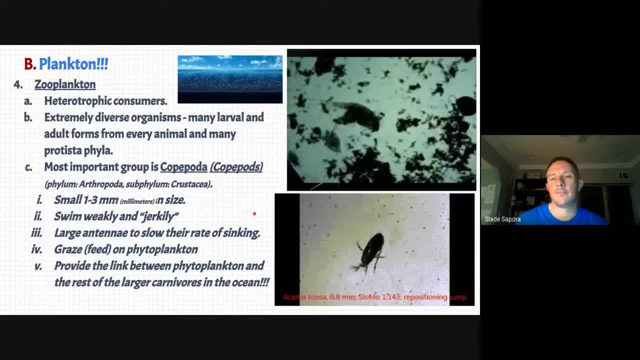 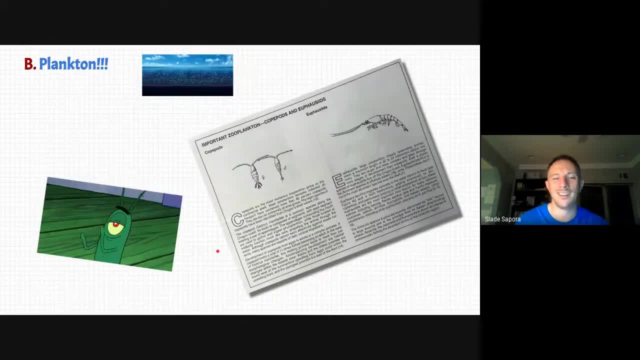 What a jerk Dude. am I done? Are we done? I think we are All right. Well, that was our lecture on plankton And I hope you enjoyed it. Read the textbook. There's the pages. Review those pages and fill out your weekly questions. 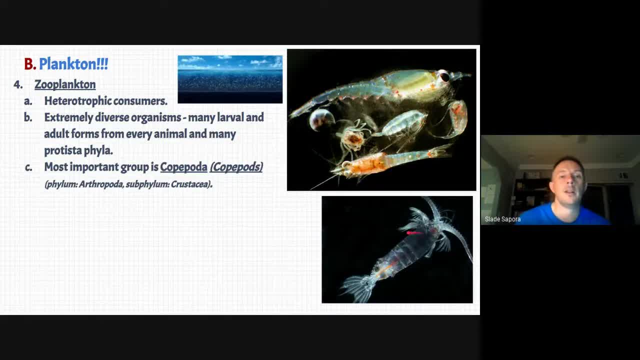 The most important group would be these copepods. Again, they're a type of a crustacean, So they're in the group Arthropoda, which is the largest group of animals on the planet, includes insects and arachnids, and millipedes and dragonflies. 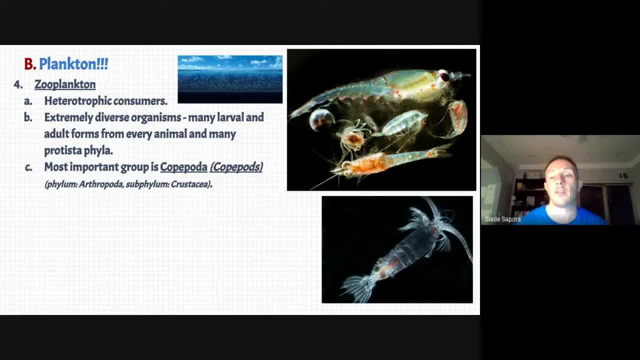 And crustaceans. crustaceans are crabs and shrimps and all these other things as well. It's a huge, huge, huge, diverse group. 80% of all planet animals are arthropods and a chunk of that are crustaceans. But just pure abundance, pure numbers. copepods- they're more numerous than 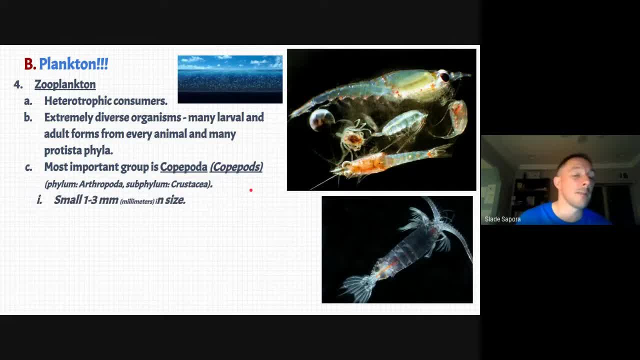 any other type of animal on the planet. They're everywhere in the oceans because they're small. So yeah, one to three millimeters in size. You can kind of see the moving in the water, but you can't really tell what it is unless you have a microscope. They swim weakly and jerkily. 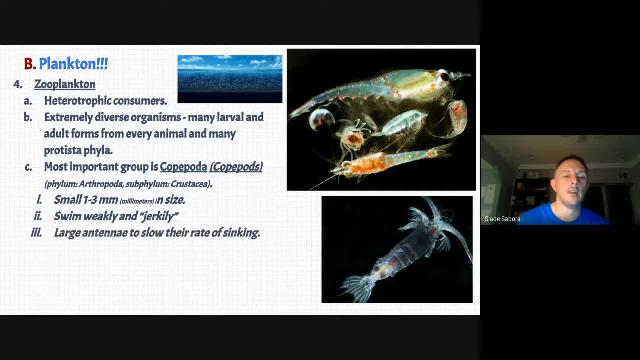 They use their little antenna to float, and they can, to help give them buoyancy. Again, large antennas slow their state of rate of sinking, And that's the same as with dendroflagellates we were just talking about. They graze and feed on phytoplankton and they 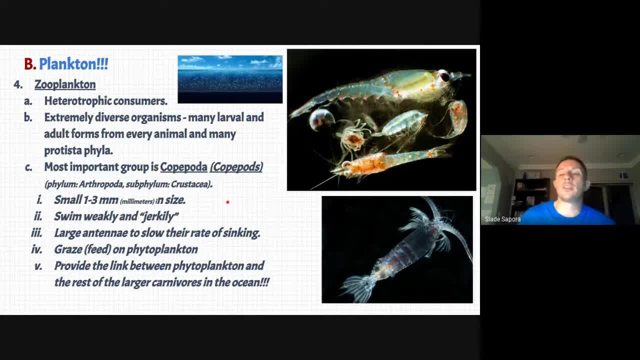 provide a link between that phytoplankton and the larger carnivores. So the things that eat the copepods, they're going to eat the copepods And they're going to eat the copepods And they're going to eat the phytoplankton. So if really the copepods weren't, there pretty much life in the 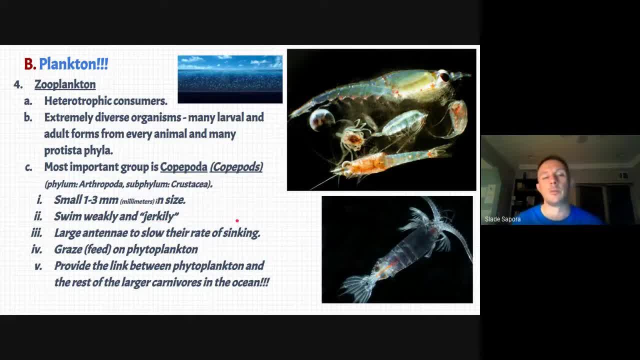 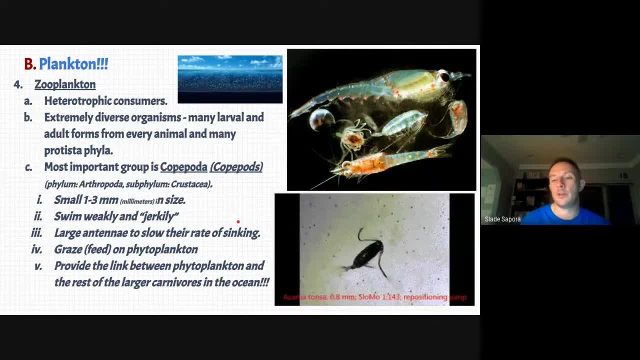 ocean would kind of stop. They are that link between those super microscopic phytoplankton and other things as well. Here's a picture of one moving jerkily through the water using their antenna. Okay, wonderful, Oh look, there's another one. What a jerk. 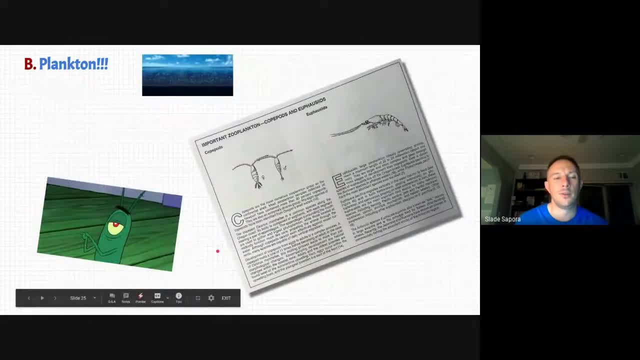 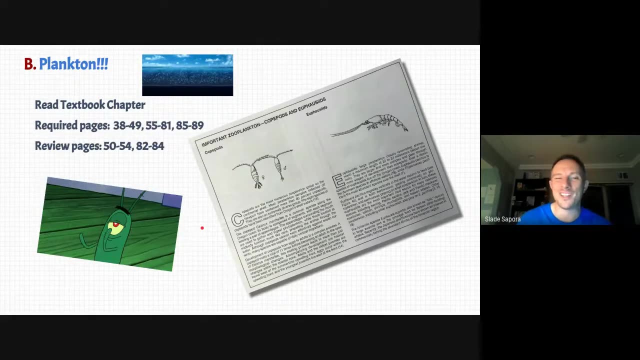 Dude, am I done? Are we done? I think we are All right. Well, that was our lecture on plankton And I hope you enjoyed it. Read the textbook. There's the pages. Review those pages and fill out your weekly questions. Next week we'll be talking about vertebrates. That's all I got. I. 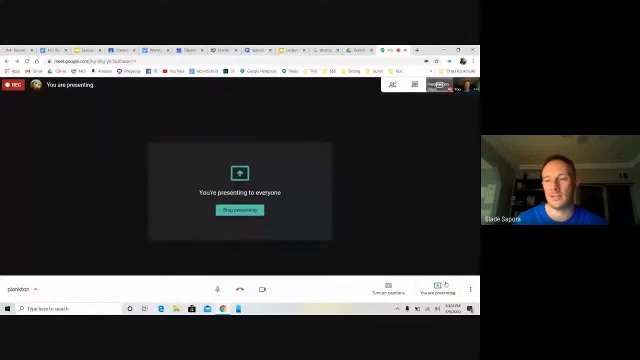 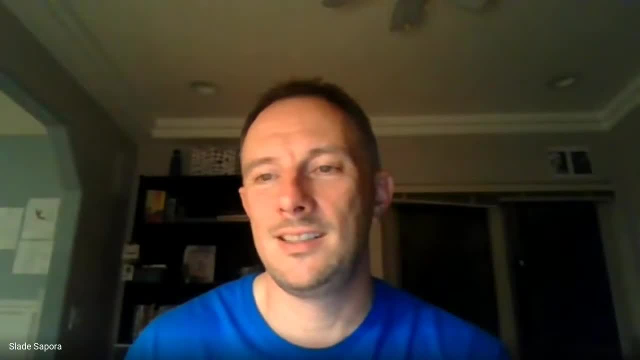 just got to figure out how to exit out of here. How long was this? And stop recording Later.